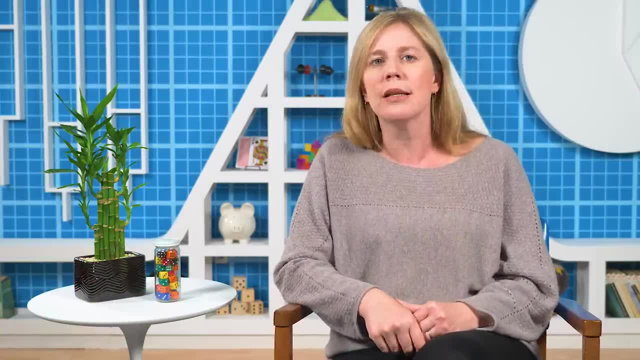 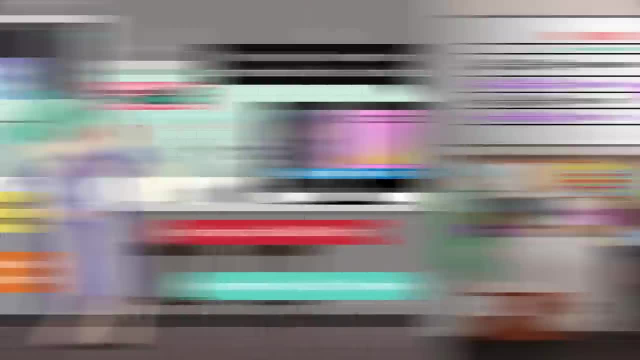 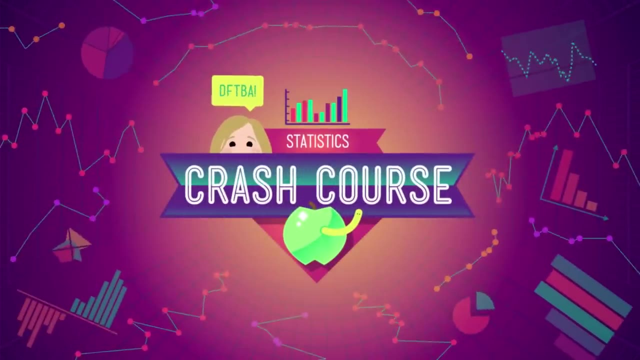 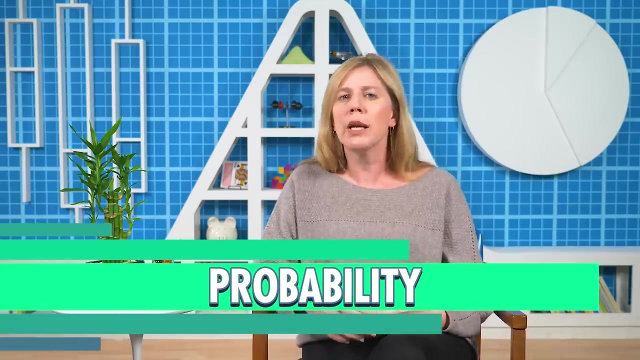 Our brains recognize patterns in everything, especially in sequences of events like the kind we're going to talk about today. as we start talking about probability, Alright, first let's just establish a more specific definition of what probability is, Because the way we use the word in everyday life can be different from how we use it in. 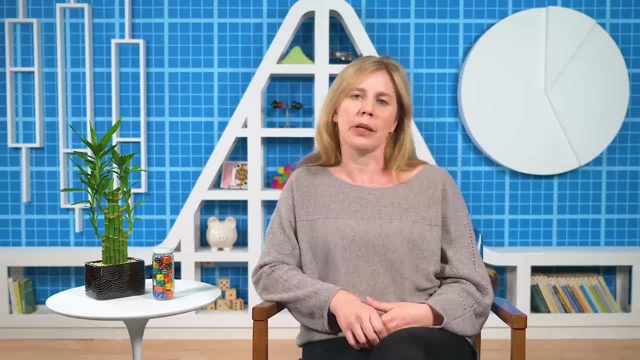 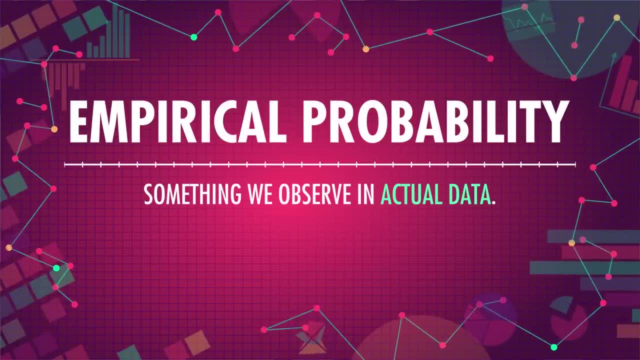 statistics. Statisticians talk about two types of probability: empirical and theoretical. Empirical probability is something we observe in actual data, like the ratio of girls in each individual family. It has some uncertainty because, like the samples in experiments, it's just a small. 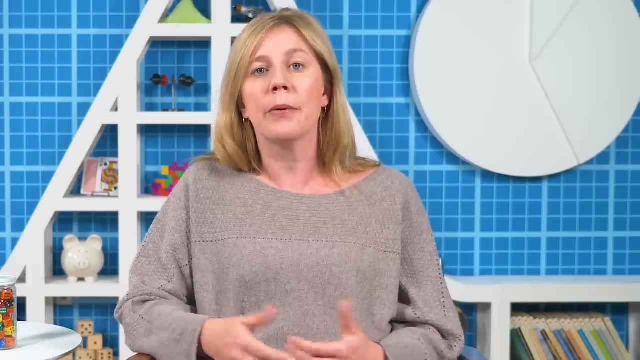 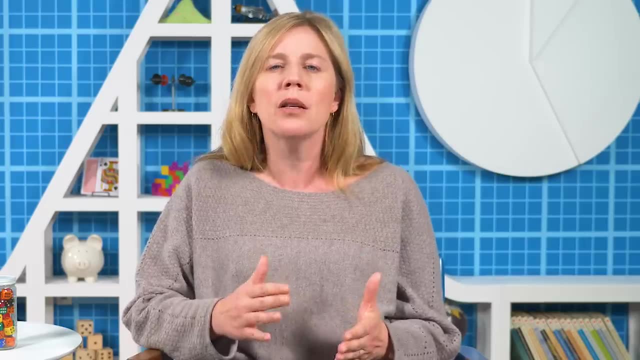 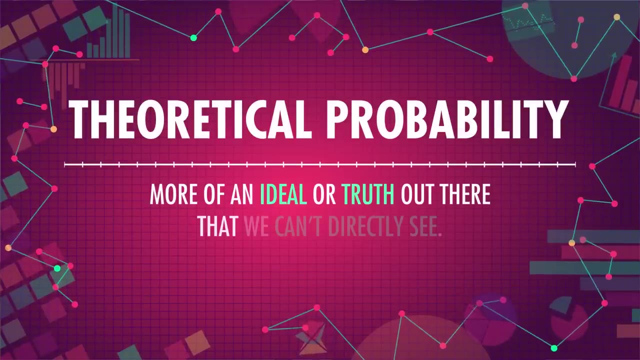 amount of the data that's available. Empirical probabilities, like sample statistics, give us a glimpse at the true theoretical probability, but they won't always be equal to it, because of the uncertainty and randomness of any sample. Theoretical probability, on the other hand, is more of an ideal or truth out there that 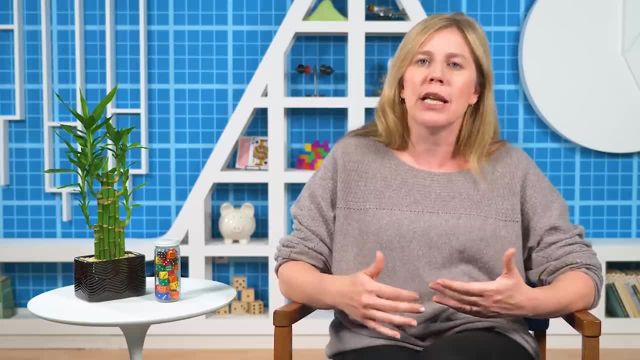 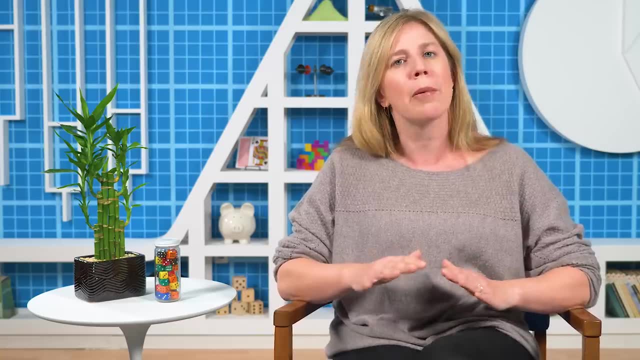 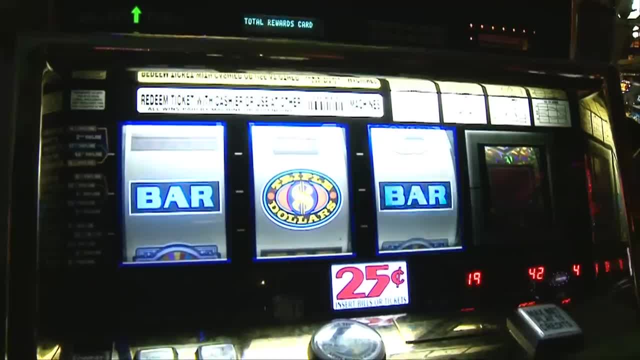 You'll be able to guess the probability of winning the jackpot by counting the number of times you win and dividing it by the number of times you played. If you play 100 times and win 6 times, you can be pretty sure that you're winning the. 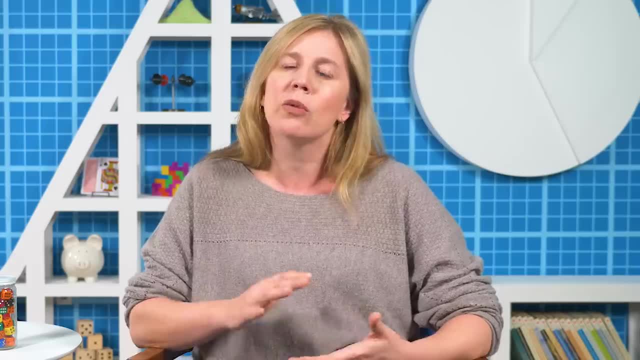 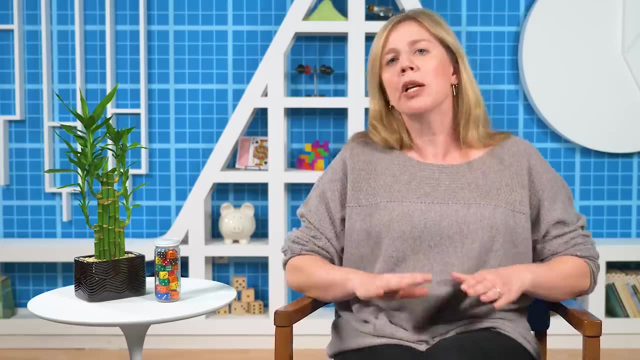 jackpot. So you're pretty sure that the probability of getting a jackpot is around 6 out of 100, or 6%. Now, this isn't to say that you can rule out that the true probability is 5% or even 10%, but you're relatively sure that it's close to 6% and not say 99%. 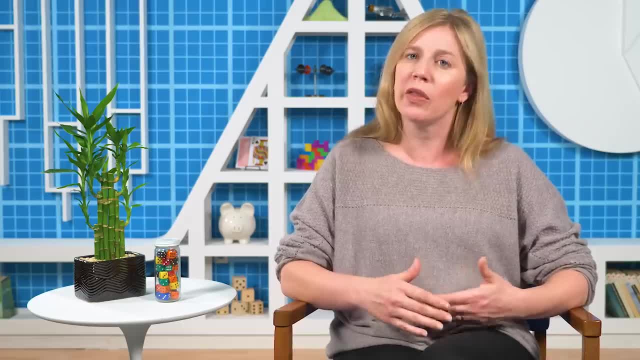 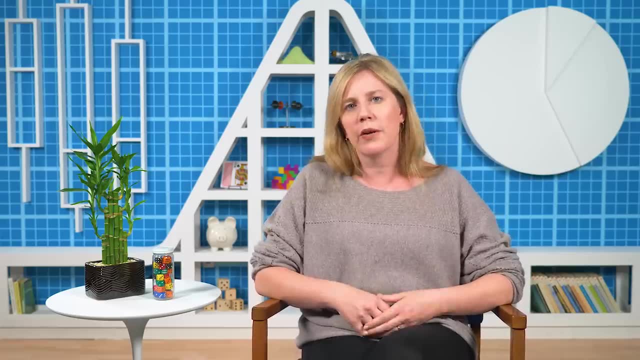 So the empirical probability can be a good estimation of the theoretical one, even if it's not exact. So far we've been talking about the probability of just one event, but often there may be two or more events that we want to consider. Like what, if you want to know the probability of picking a purple or a red? 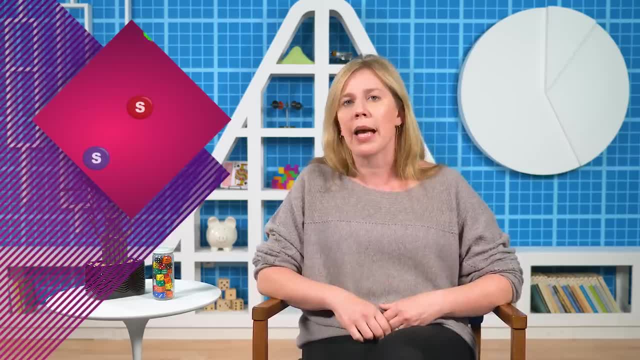 Well, that's a good question, And if you want to know the probability of picking a purple or a red, you can use the probability of picking a purple or a red skittle from a bag. The proportion of each color in a bag of skittles is roughly equal: 20% for each of the 5 colors. 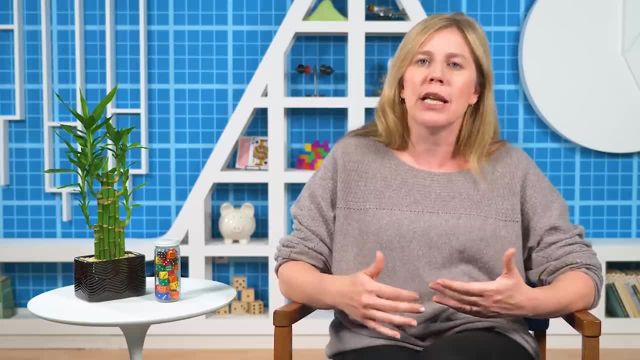 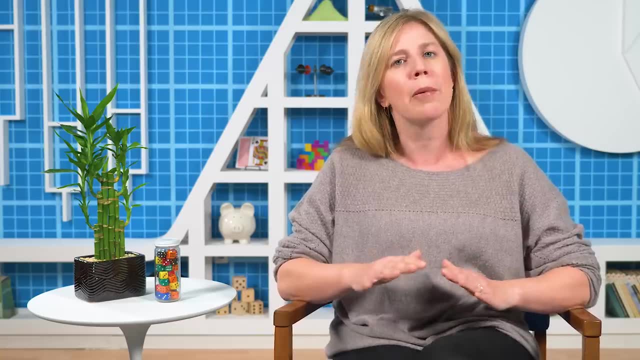 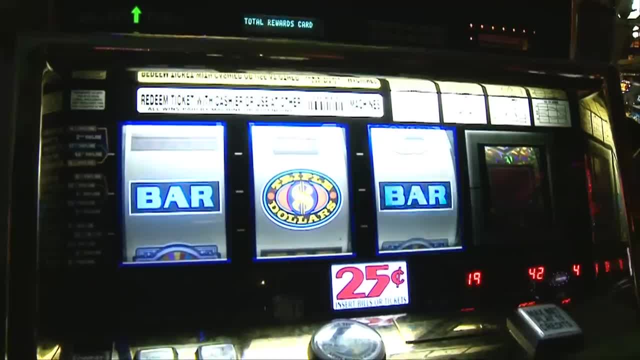 You'll be able to guess the probability of winning the jackpot by counting the number of times you win and dividing it by the number of times you played. If you play 100 times and win 6 times, you can be pretty sure that you're winning the. 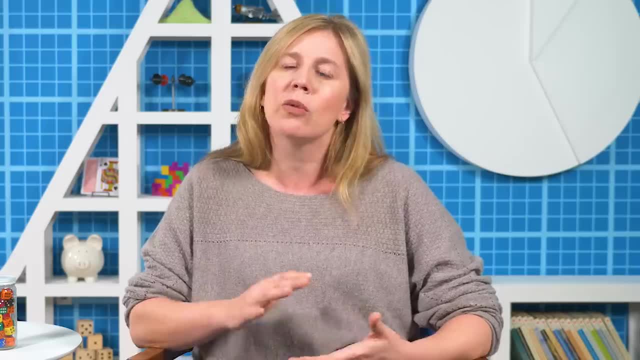 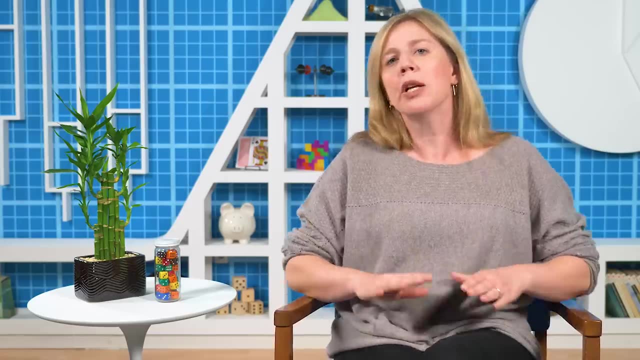 jackpot And you're pretty sure that the probability of getting a jackpot is around 6 out of 100, or 6%. Now, this isn't to say that you can rule out that the true probability is 5% or even 10%, but you're relatively sure that it's close to 6% and not, say, 99%. 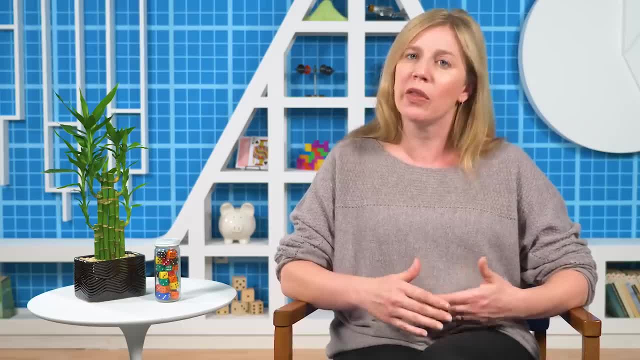 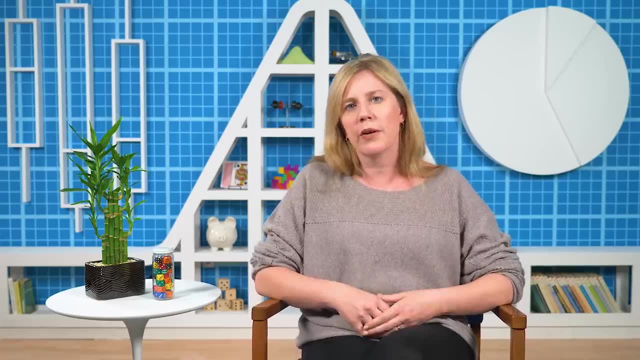 So the empirical probability can be a good estimation of the theoretical one, even if it's not exact. So far we've been talking about the probability of just one event, but often there may be two or more events that we want to consider. Like what, if you want to know the probability of picking a purple or a red? Well, if you're a jackpot, you're probably going to want to know the probability of picking a purple or a red, And if you're a jackpot, you're probably going to want to know the probability of picking a purple or a red. Well, if you're a jackpot, you're probably going to want to know the probability of picking a purple or a red, And if you're a jackpot, you're probably going to want to know the probability of picking a purple or a red. 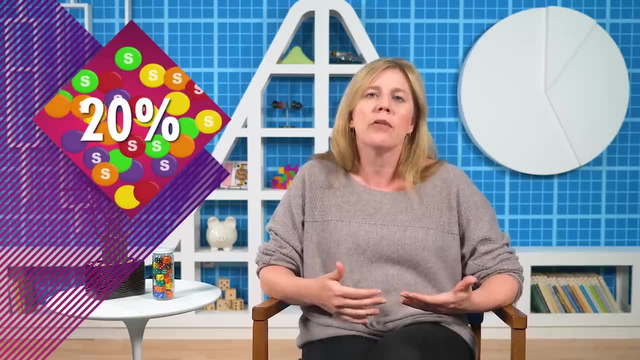 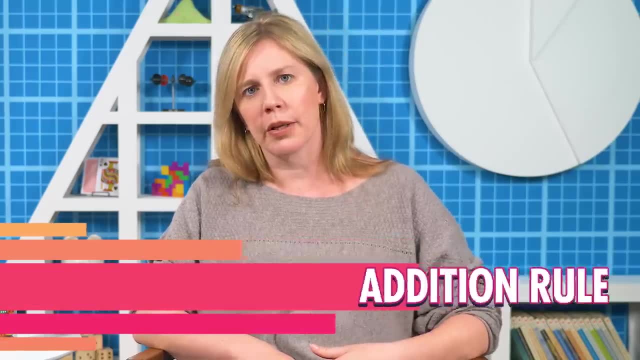 The proportion of each color in a bag of Skittles is roughly equal 20% for each of the 5 colors. So let's say you randomly select a Skittle without looking. For this we need the addition rule of probability. 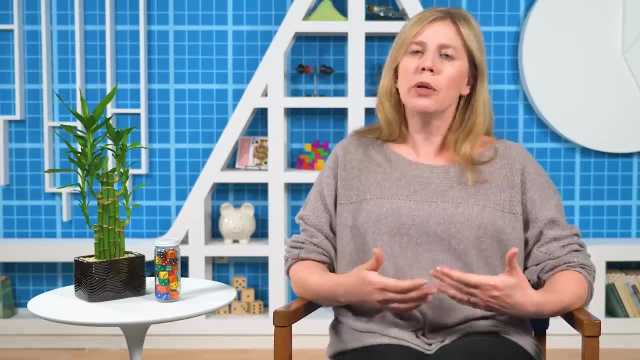 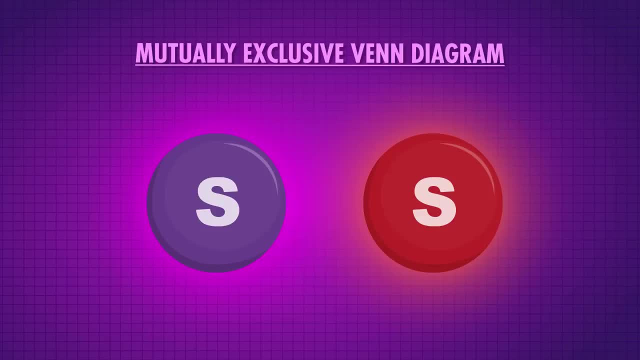 Since a Skittle can't be two different colors at once, the color possibilities are mutually exclusive. That means the probability of a Skittle being red and purple at the same time is zero. So we can use the simplified addition rule, which says that the probability of getting 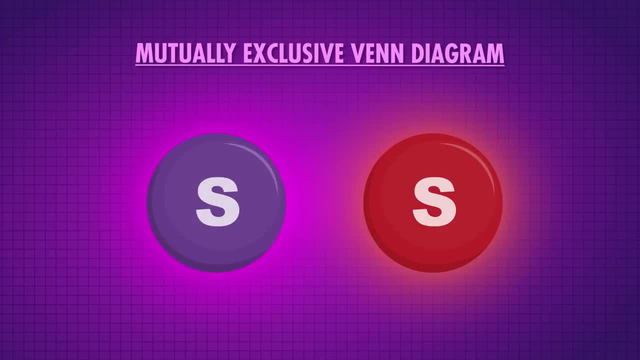 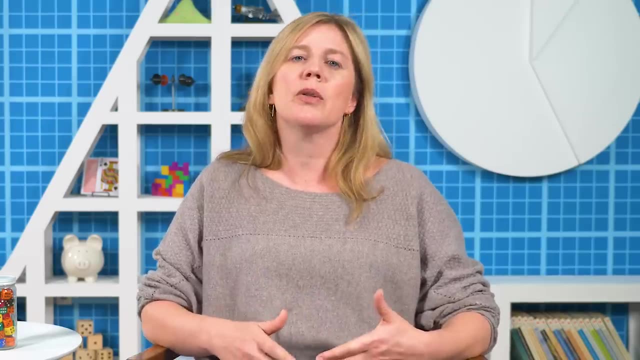 a red or purple Skittle is the sum of the probability of getting a red or purple Skittle and the probability of getting a purple Skittle. Since we're going to be talking a lot about probability in the next few episodes, I'm going to introduce a little notation. 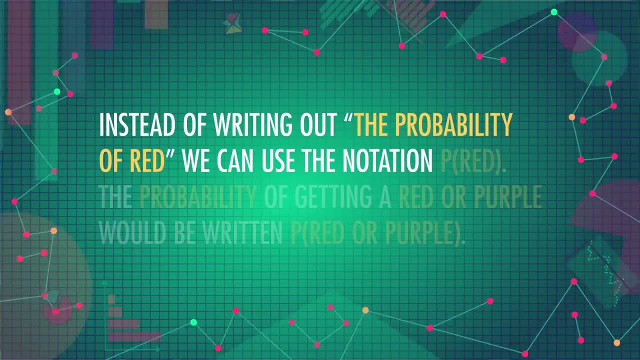 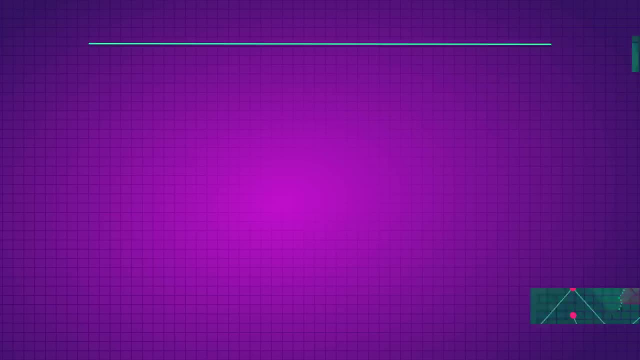 Instead of writing out the probability of red, we can use the notation P of red. The probability of getting a red or purple would be written P of red or purple. So far we know what the probability of red or purple is. It's P of red plus P of purple, or .2 plus .2.. 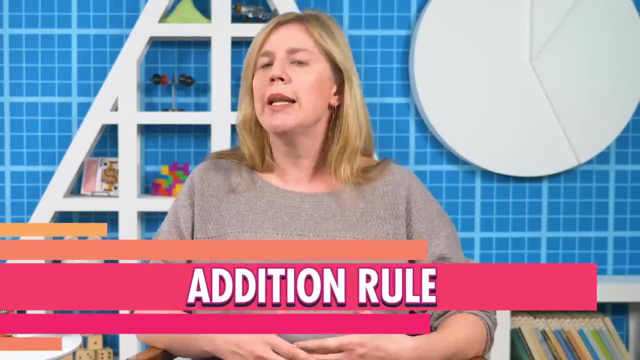 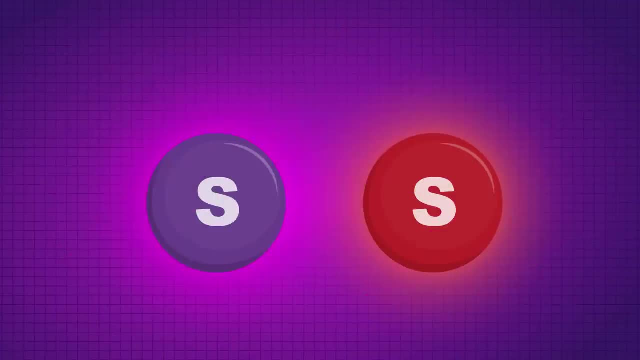 So let's say you randomly select a skittle without looking. For this, we need the addition rule of probability. Since a skittle can't be two different colors at once, the color possibilities are mutually exclusive. That means the probability of a skittle being red and purple at the same time is zero. 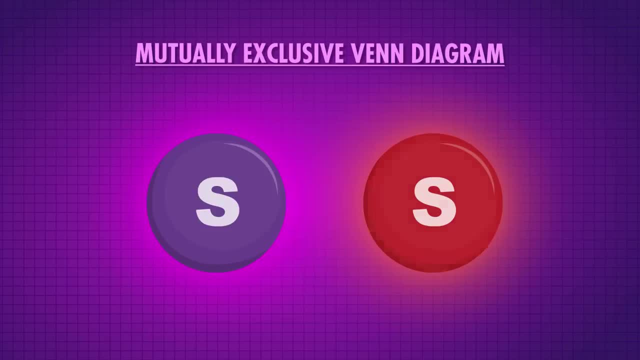 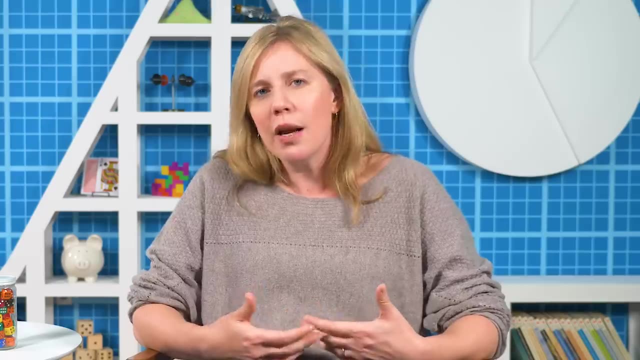 So we can use the simplified addition rule, which says that the probability of getting a red or purple skittle is the sum of the probability of getting a red or a purple skittle and the probability of getting a purple. Since we're going to be talking a lot about probability in the next few episodes, I'm 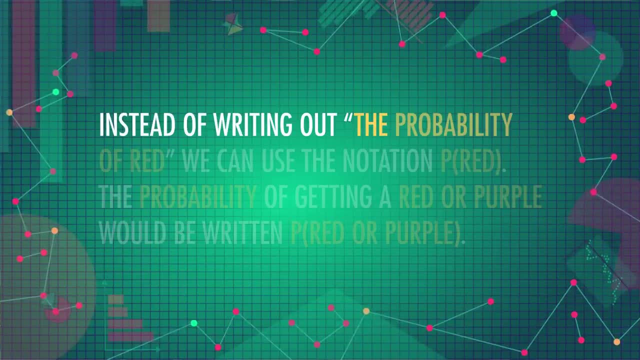 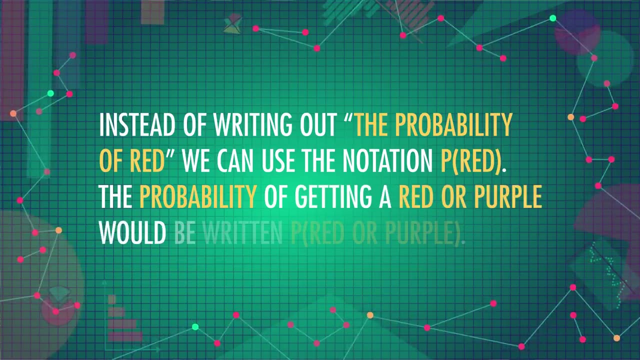 going to introduce a little notation. Instead of writing out the probability of red, we can use the notation p of red. The probability of getting a red or purple would be written p of red or purple. So far we know what the probability of red or purple is. 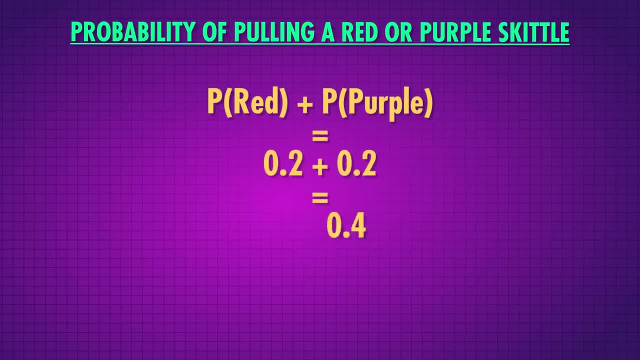 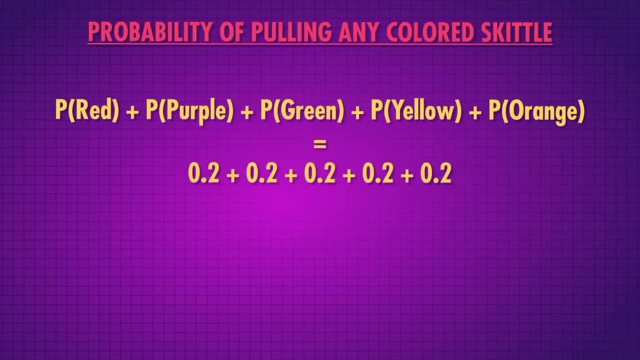 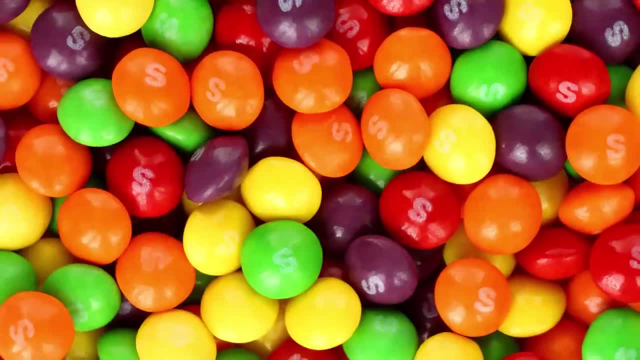 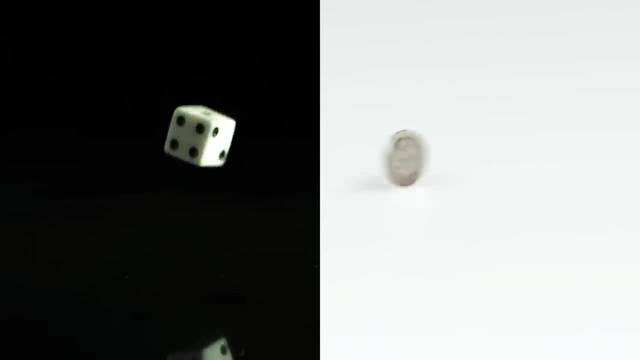 0.2.. That's 100% Good odds. Red and purple skittles are mutually exclusive, but not all the events we're interested in are. For example, if you roll a die and flip a coin, the probability of getting tails is. 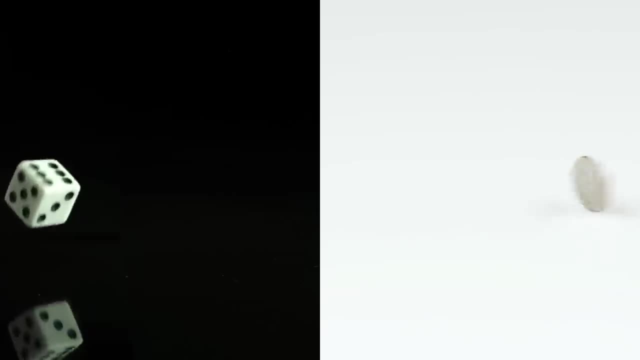 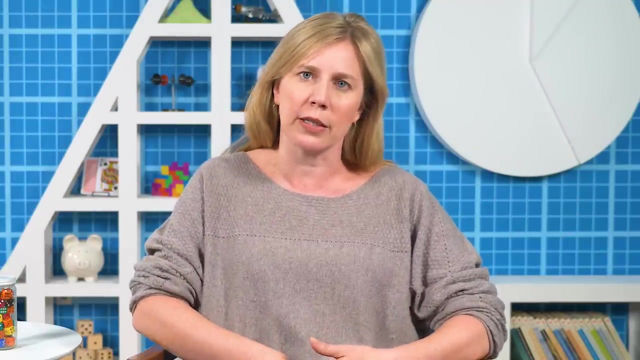 not mutually exclusive of rolling a six, since you can both roll a six and flip tails in the same turn. Since p of tails or six is not equal to zero, these two events are not mutually exclusive And we'll need to adjust our addition rule accordingly. 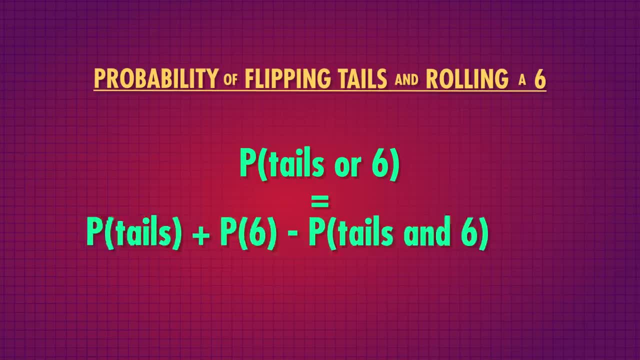 The full version of the addition rule states that p of tails or six equals p of tails plus p of six, minus p of tails and six. When two things are mutually exclusive, the probability that they happen together is zero. so we ignored it. 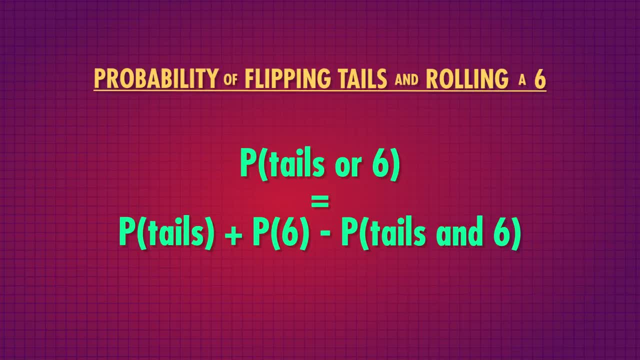 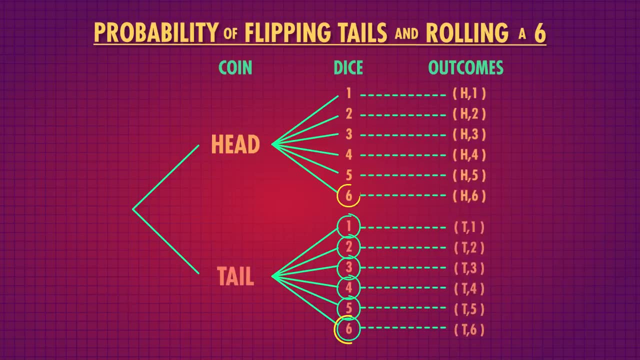 But now the probability of both these things happening is not zero, so we need to calculate it. You can see here there are 12 possible outcomes when flipping a coin and rolling a die. There are six outcomes with tails and two outcomes with a six. 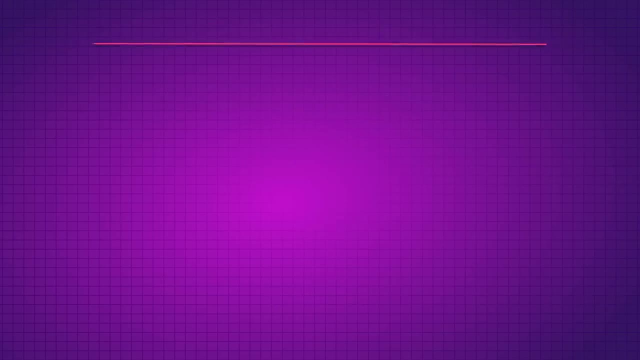 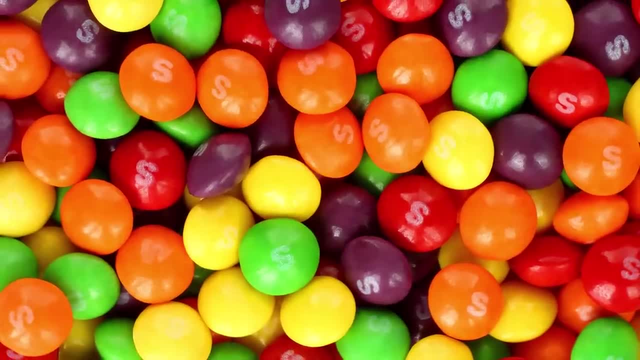 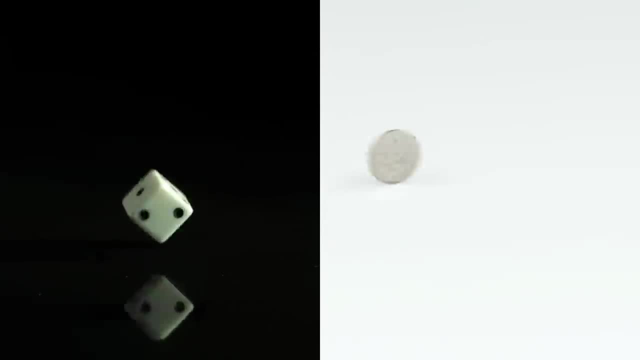 That's 100% Good odds. Red and purple Skittles are mutually exclusive, but not all the events we're interested in are. For example, if you roll a die and flip a coin, the probability of getting tails is not mutually exclusive of rolling a six, since you can both roll a six and flip tails. 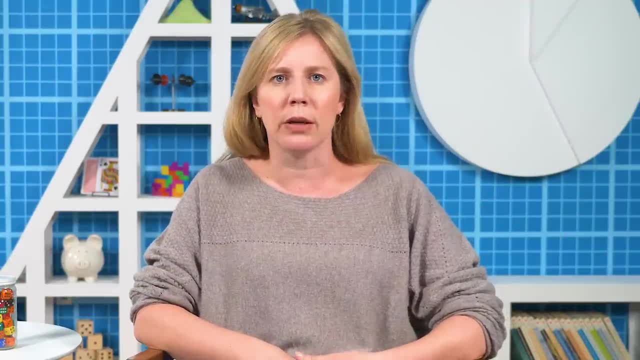 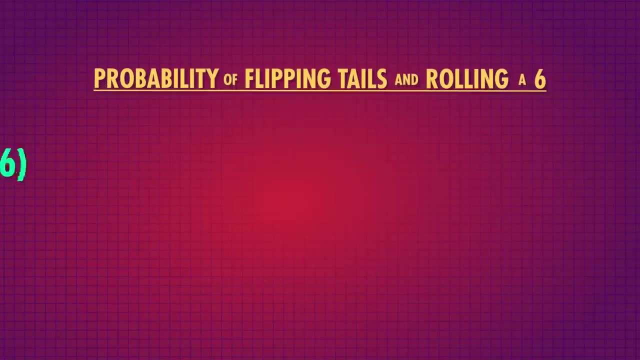 in the same turn. Since P of tails or six is not equal to zero, these two events are not mutually exclusive and we'll need to adjust our addition rule accordingly. The full version of Skittles is zero. The full version of the addition rule states that P of tails or six equals P of tails plus. 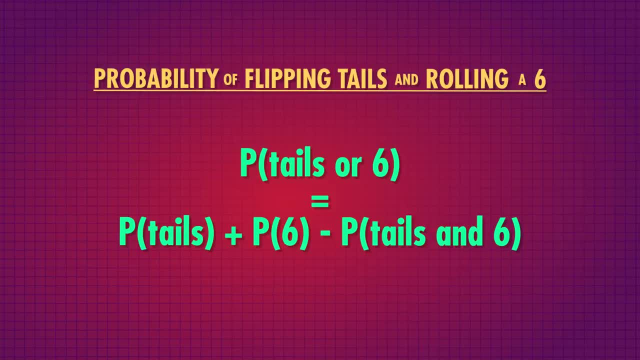 P of six minus P of tails and six. When two things are mutually exclusive, the probability that they happen together is zero, so we ignored it. But now the probability of both these things happening is not zero, so we need to calculate it. 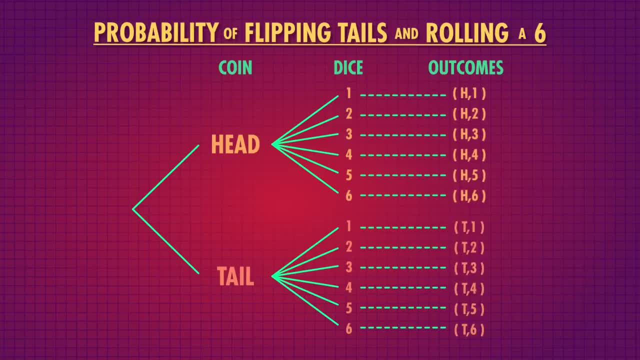 You can see here, there are 12 possible outcomes when flipping a coin and rolling a die. There are six outcomes with tails and two outcomes with a six. If we add all of those together we get eight. But by looking through the chart we can tell that there are only seven possible outcomes. 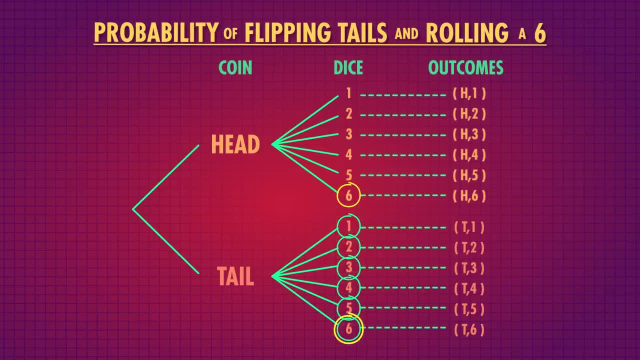 that have either tails or a six. When we count tails and sixes independently, we double count the outcomes that have both. If we didn't subtract off the probabilities of tails and six, we would double count it. Let's put these probabilities into a Venn diagram and we can see even more clearly. 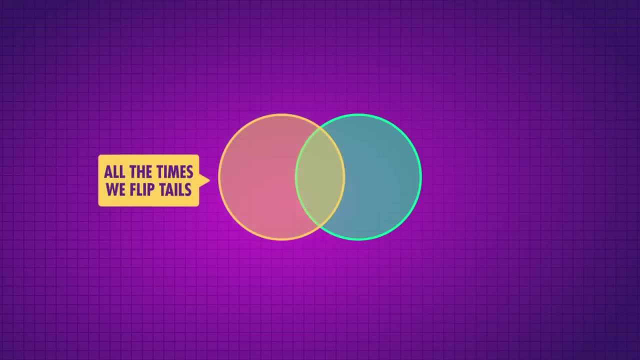 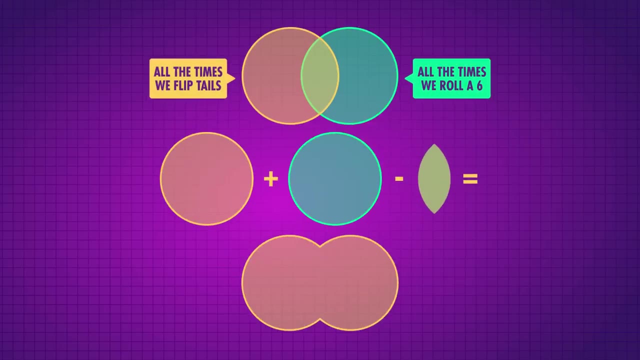 why we need to subtract P of tails and six If this circle is all the times we flip tails and the other circle is all the times we roll a six ETEX EXCELORES is counted twice if we simply added the two circles together. 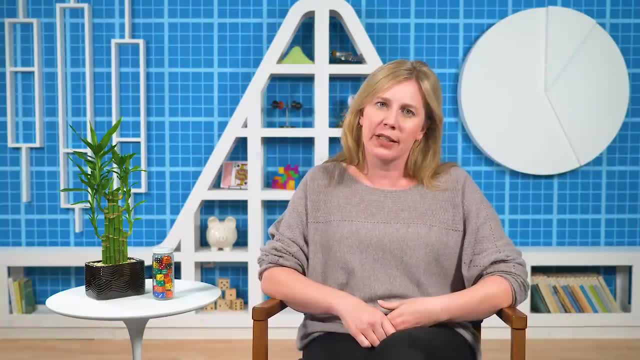 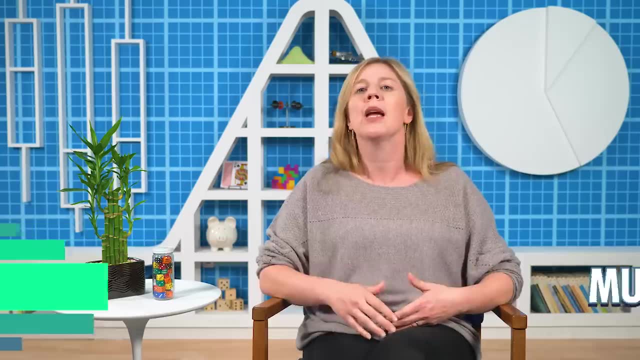 In this simple case, we could easily see what the probability of tails and six is. but sometimes it's not so easy to figure out. That's why we have the multiplication rule, which helps us figure out the probability of two or more things happening at the same time. 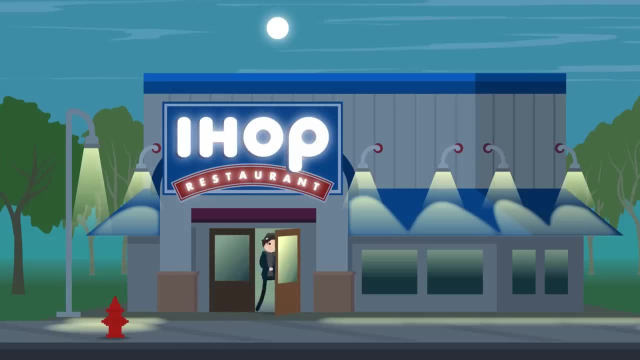 Let's say, you just found out that actor Cole Sprouse goes to your local IHOP pretty often and there's a 20% chance he'll be there for dinner any given night. And yeah, I know that's not how people work. 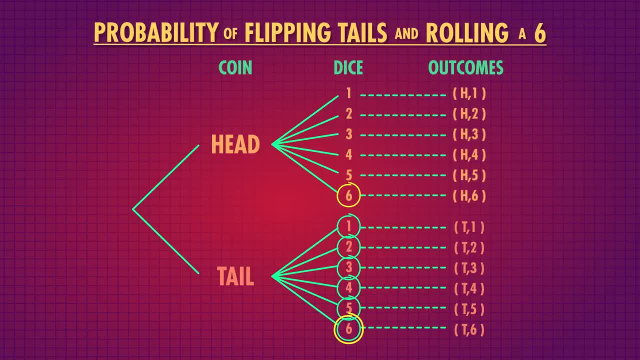 If we add all of those together we get zero. So we need to calculate it. But by looking through the chart we can tell there are only seven possible outcomes that have either tails or a six. When we count tails and sixes independently, we double count the outcomes that have both. 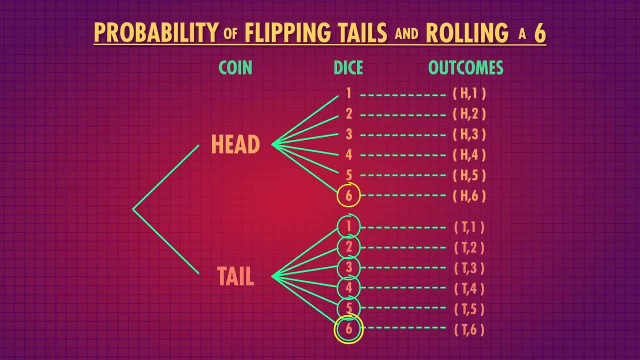 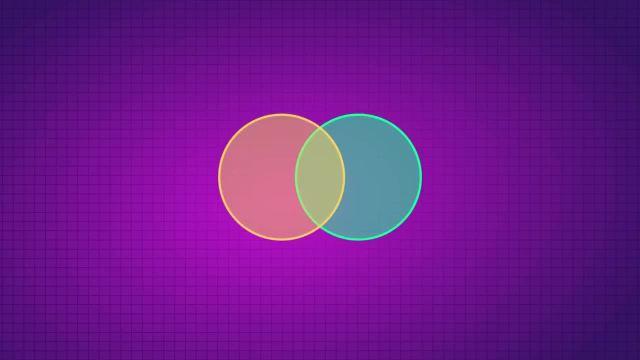 If we didn't subtract off the probabilities of tails and six, we would double count it. Let's put these probabilities into a Venn diagram and we can see even more clearly why we need to subtract p of tails and six, If this circle is all the times we flip tails and the other circle is all the times we roll. 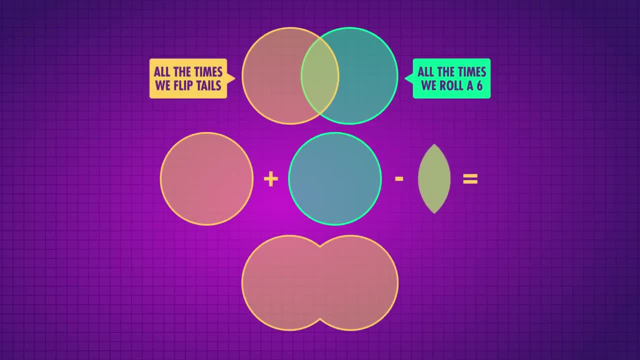 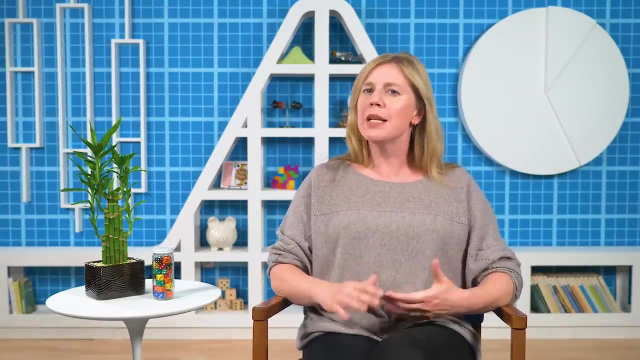 a six, The overlapping area is counted twice. if we simply added the two circles together In this simple case, we could easily see what the probability of tails and six is. but sometimes it's not so easy to figure out. That's why we have the multiplication rule, which helps us figure out the probability. 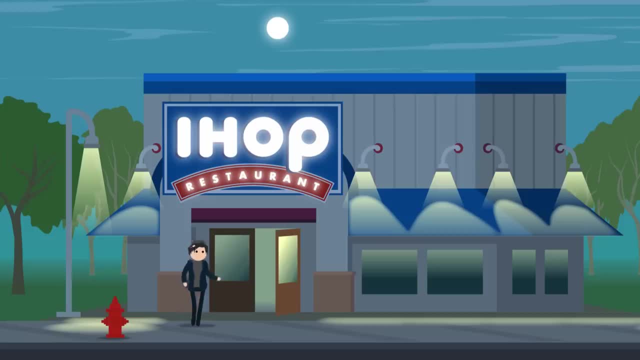 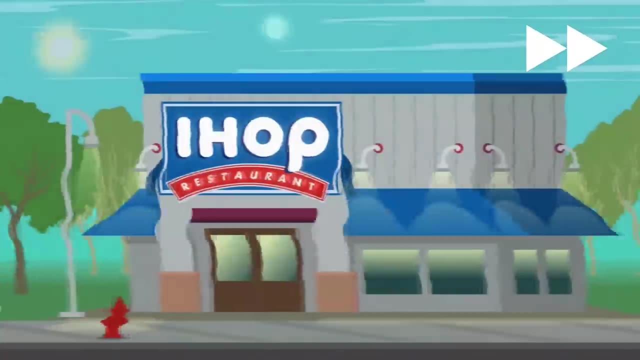 of two or more things happening at the same time. Let's say, you just found out that actor Cole Sprouse goes to your local IHOP pretty often and there's a 20% chance he'll be there for dinner any given night. 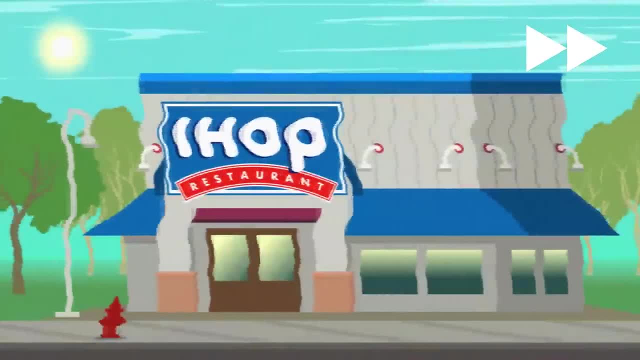 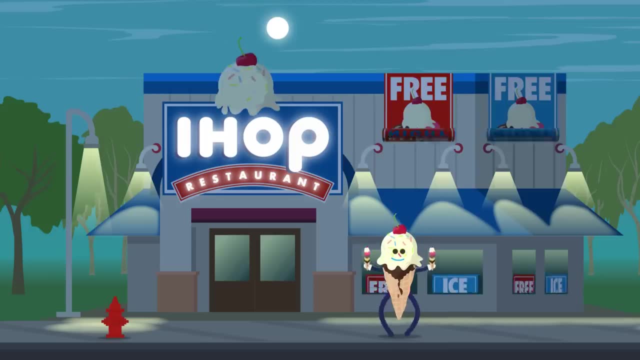 And yeah, I know that's not how people work, but we're going to say that's how Cole Sprouse works. Anyway, to top that off, your local IHOP has a promotion where they randomly select certain nights to be free ice cream nights, in the hopes that customers will keep coming. 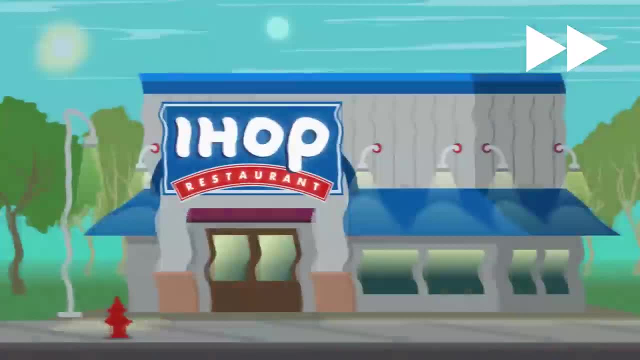 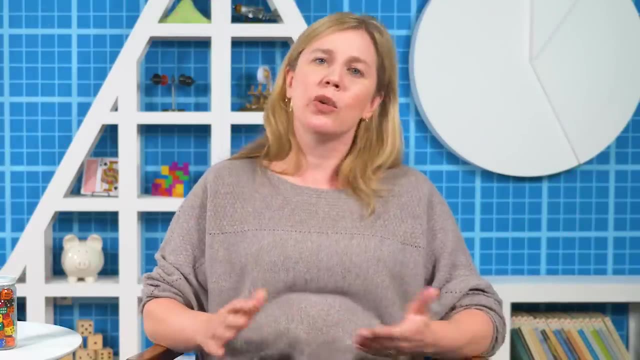 back in case that night is the night Each night. there's a 10% chance that it will be free ice cream night. Now, you love ice cream and you like like Cole Sprouse, as do we all, and your perfect night would include them both. 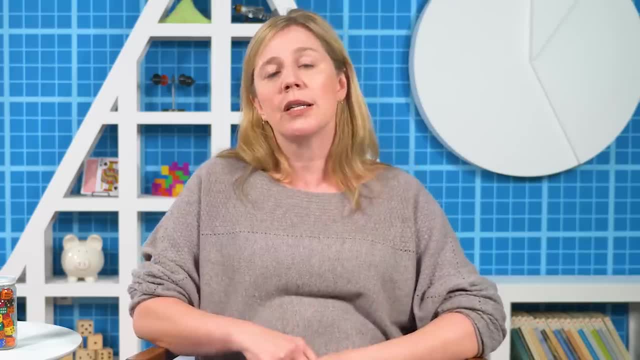 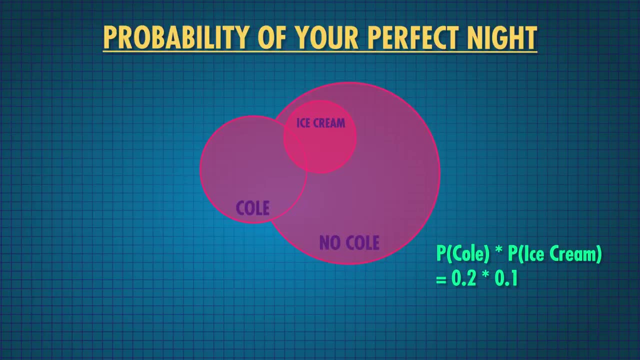 So you try to calculate the probability that will happen on your visit tonight Using the multiplication rule, Identify the probability that Cole Sprouse will be at the IHOP with the probability that it will be free ice cream night, and you come to the sad realization: there's. 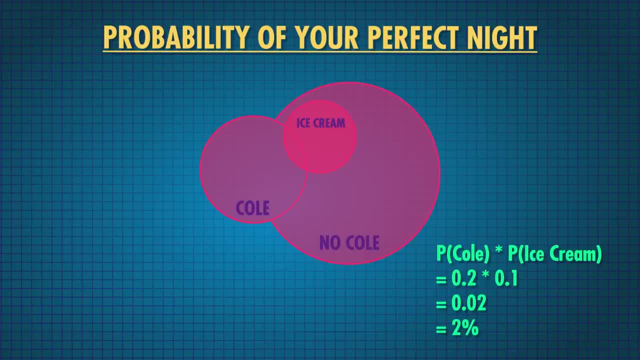 only a 2% chance that you'll get to see Cole and get free dessert tonight. When we want to know the probability of two things happening at the same time, we first need to look at only the times when one thing- Cole Sprouse at IHOP- is true, which is 20%. 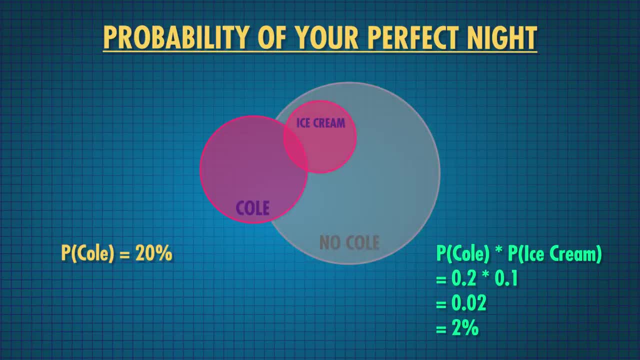 of the time. Now that we've reduced our options to just Cole nights, out of all of those Cole times, how often is it free ice cream time? Only 10% of Cole nights, 10% of the original 20%, leaves only a 2% chance that both will. 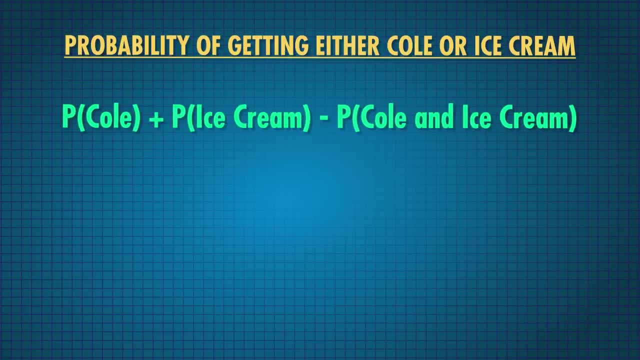 happen at the same time, But you can always change your expectations and calculate the probability of getting either by using the addition rule, Cole or free ice cream, which is calculated by adding the probability of Cole to the probability of free ice cream, minus the probability of both. 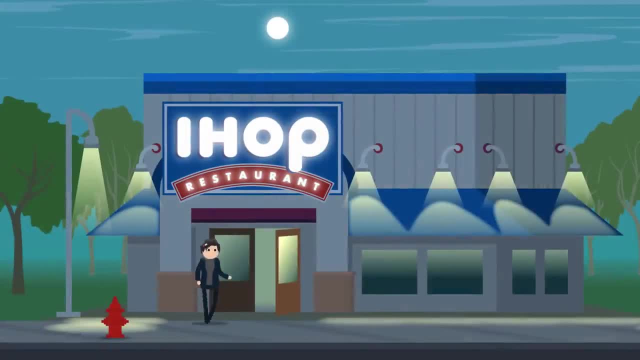 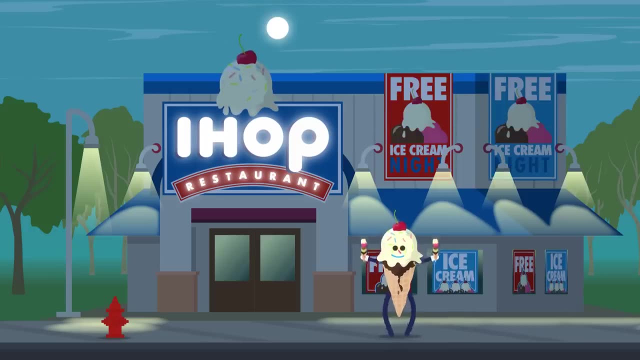 but we're gonna say that that's how Cole Sprouse works. Anyway, to top that off, your local IHOP has a promotion where they randomly select certain nights to be free ice cream nights, in the hopes that customers will keep coming back, in case that night is the night. 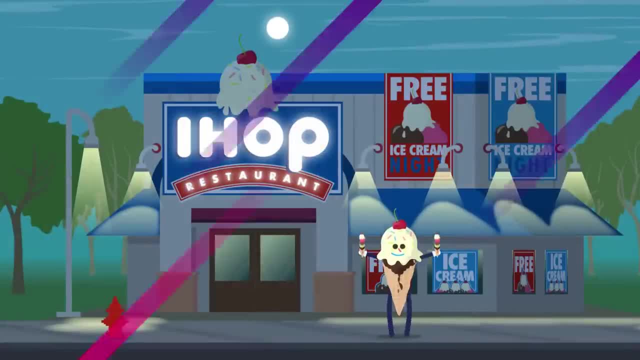 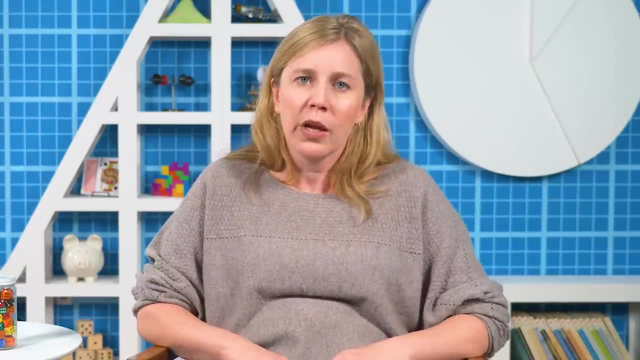 Each night, there's a 10% chance that it will be free ice cream night. Now, you love ice cream and you like like Cole Sprouse, as do we all, and your perfect night would include them both. So you try to calculate the probability. 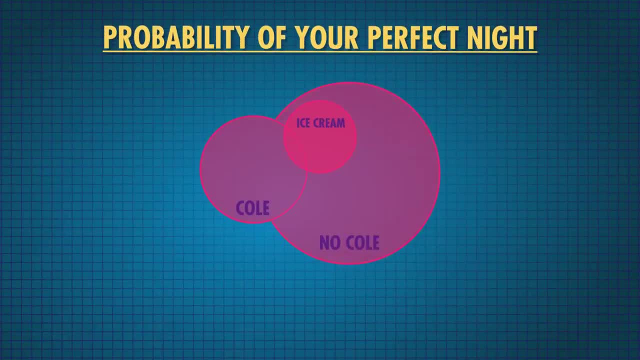 that will happen on your visit tonight. Using the multiplication rule, multiply the probability that Cole Sprouse will be at the IHOP- point two- with the probability that it will be free ice cream night- point one- and you come to the sad realization. 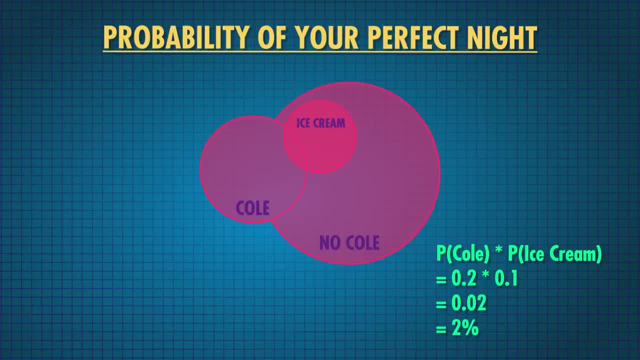 there's only a 2% chance that you'll get to see Cole and get free dessert tonight. When we wanna know the probability of two things happening at the same time, we first need to look at only the times when one thing- Cole Sprouse at IHOP- is true. 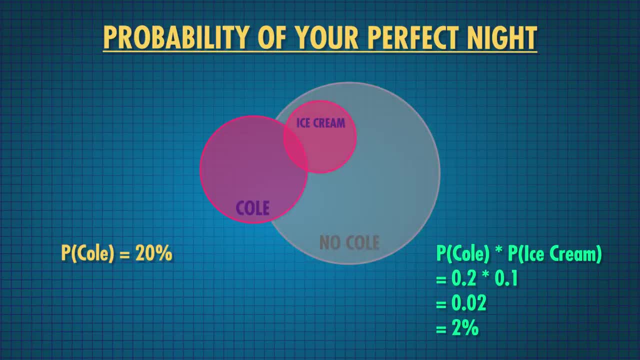 which is 20% of the time. Now that we reduced our options to just Cole nights. out of all of those Cole times, 20% of the time is free ice cream time. Only 10% of Cole nights, 10% of the original 20%. 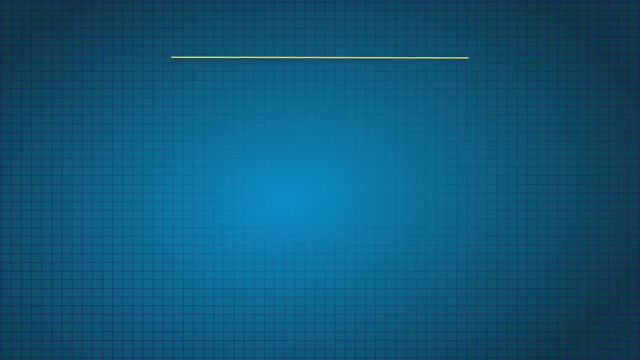 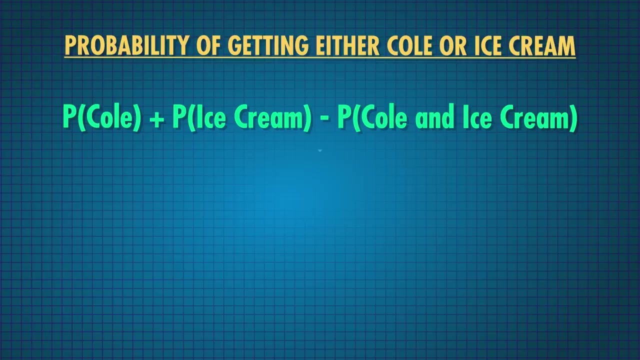 leaves only a 2% chance that both will happen at the same time, But you can always change your expectations and calculate the probability of getting either by using the addition rule Cole or free ice cream, which is calculated by adding the probability of Cole. 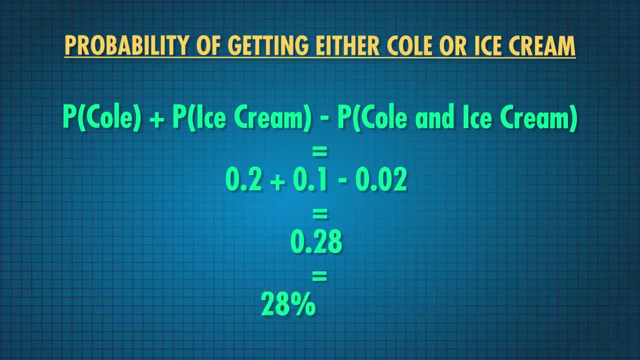 to the probability of free ice cream minus the probability of both. so we don't double count anything. You realize there's a 28% chance that something good will happen tonight. So you decide to go After what you're gonna get: French toast. 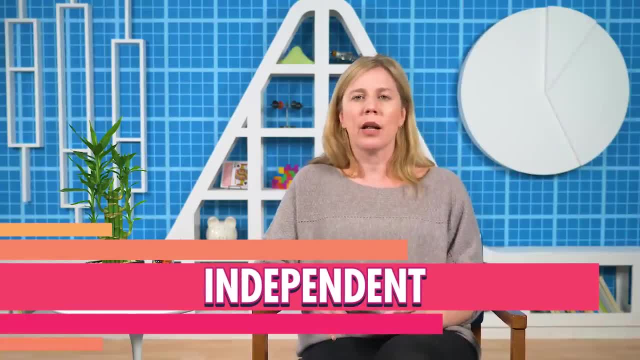 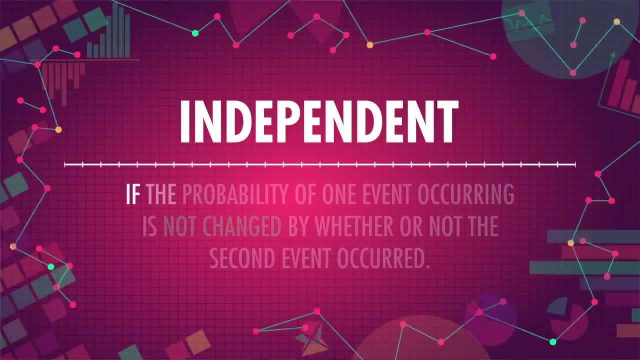 Cole Sprouse and free ice cream night are independent. Cole doesn't have any secret knowledge about when is free ice cream night, so it has never affected his decision to come. Two events are considered independent if the probability of one event occurring is not changed by whether or not the second event occurred. 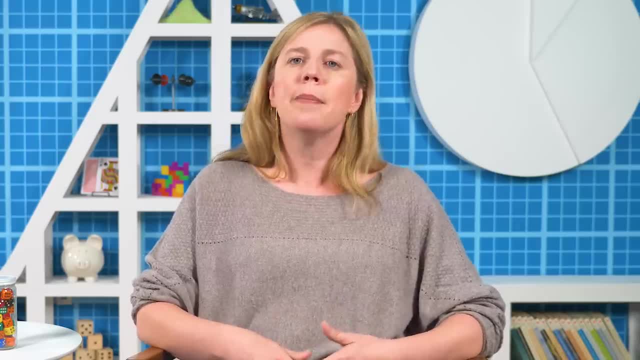 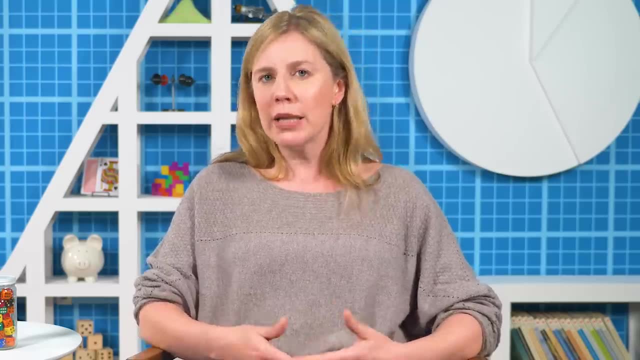 In more concrete terms, if Cole's decision to go to IHOP is independent of IHOP's decision to give out free ice cream, then the probability of Cole showing up should be the same on both ice cream and non-ice cream nights, since he's just choosing randomly. 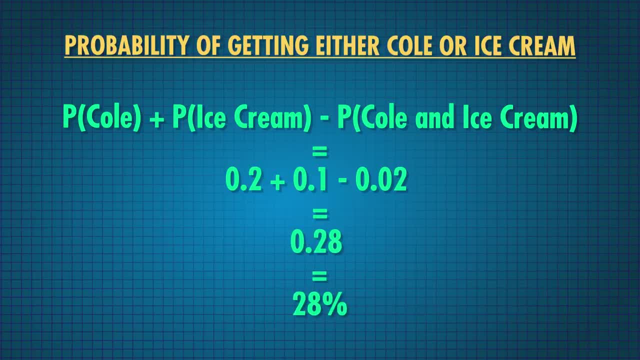 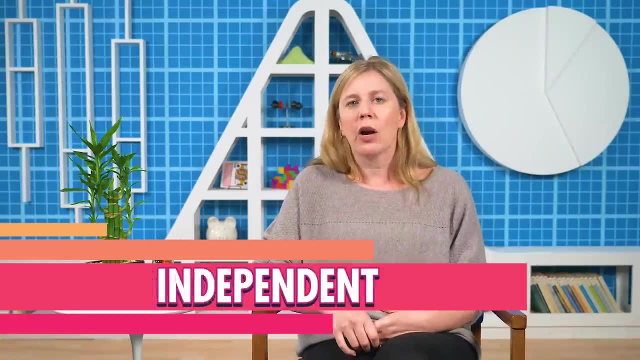 So we don't double count anything. You realize there's a 28% chance that something good will happen tonight. Here we go, No matter what you're going to get. french toast, Cole Sprouse and free ice cream night are independent. 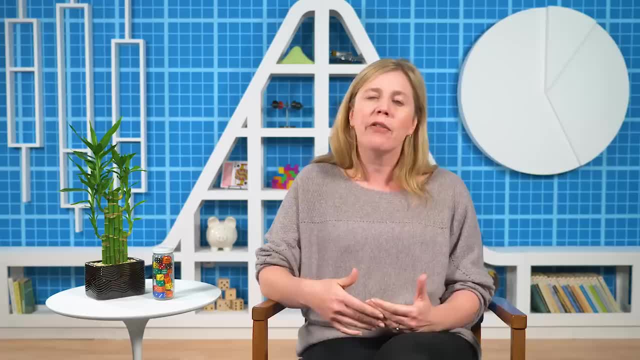 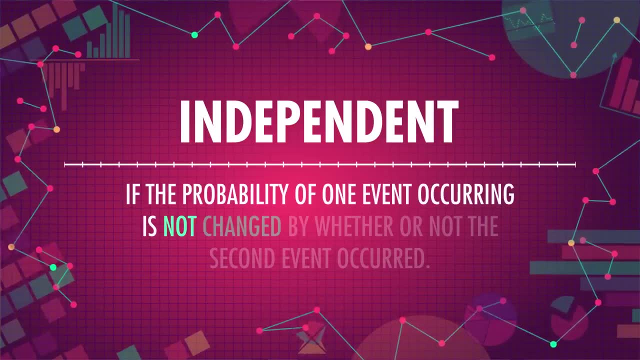 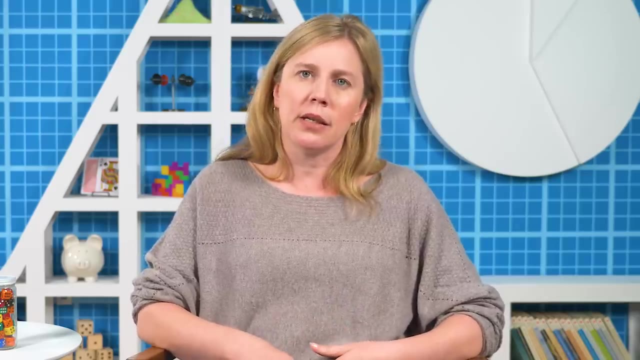 Cole doesn't have any secret knowledge about when is free ice cream night, so it has never affected his decision to come. Two events are considered independent if the probability of one event occurring is not changed by whether or not the second event occurred. In more concrete terms, if Cole's decision to go to IHOP is independent of IHOP's decision. 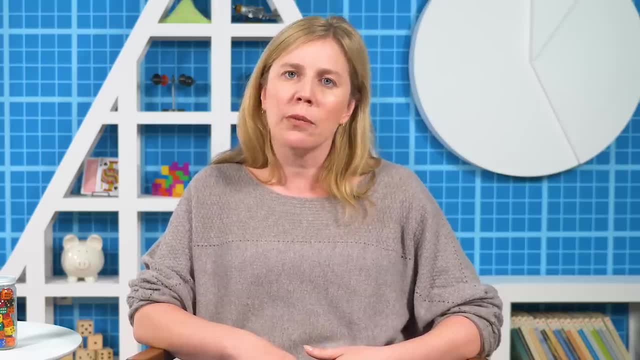 to give out free ice cream, then the probability of Cole showing up should be the same on both ice cream and free ice cream. If Cole's decision to go to IHOP is independent of IHOP's decision to give out free ice cream, then the probability of Cole showing up should be the same on both ice cream and. 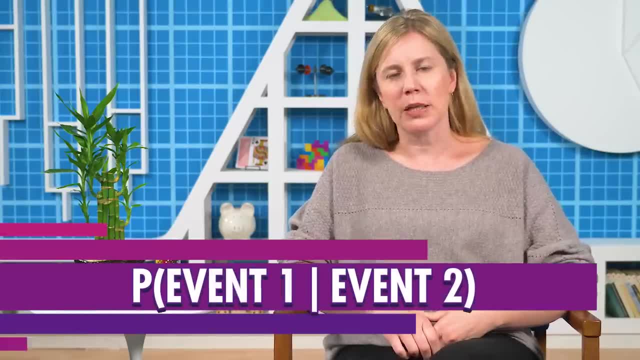 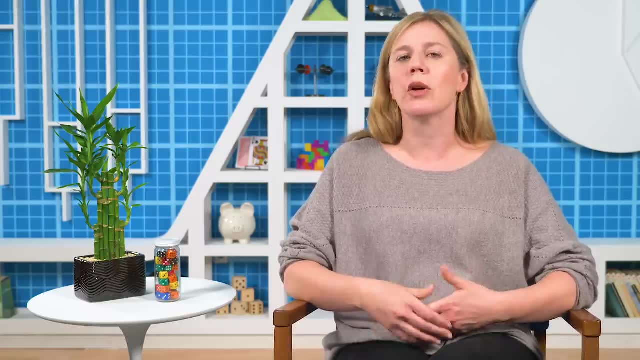 non-ice cream nights. since he's just choosing randomly, We write conditional probabilities as P of event 1, given event 2.. Conditional probabilities tell us the probability of event 1, given that event 2 has already happened. If two events are independent, like Cole and ice cream night, then we expect P of Cole. 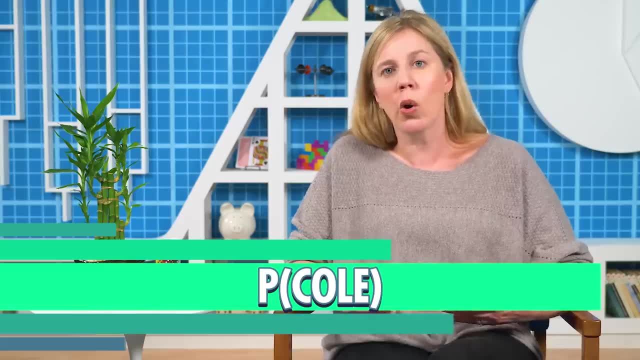 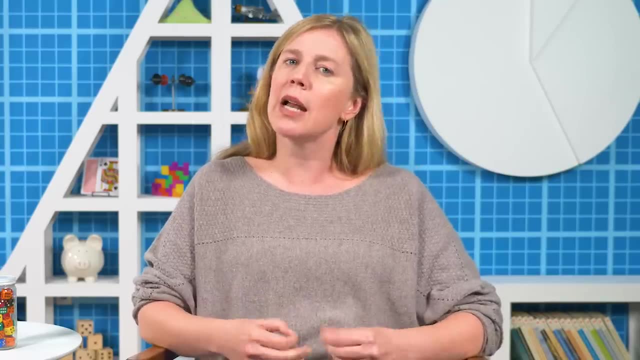 given ice cream night to be the same as just plain old P of Cole. since the two things are unrelated: If P of Cole given ice cream wasn't the same as plain old P of Cole, that means that ice cream night might somehow affect Cole's decision to show up at IHOP. 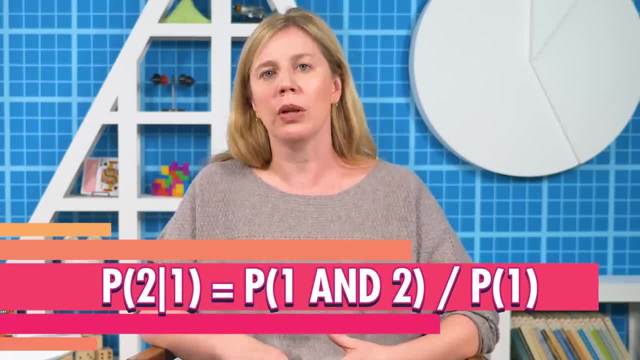 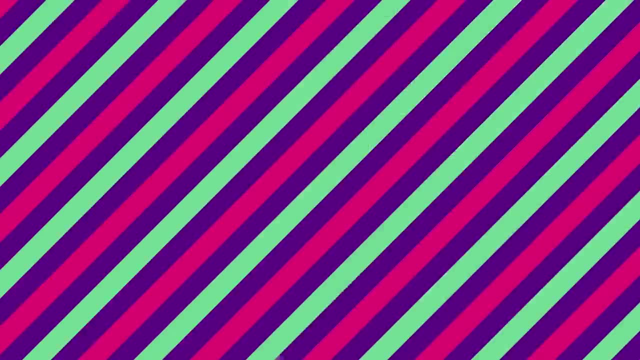 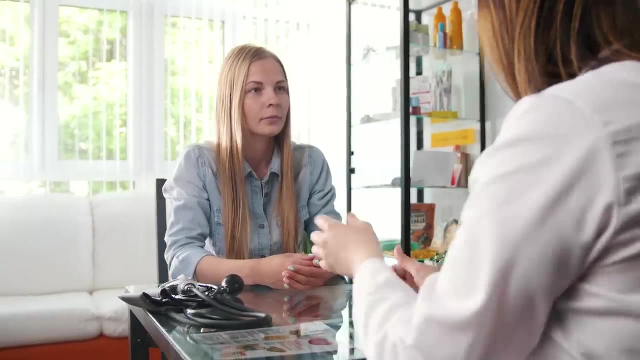 We calculate conditional probability P of event 2- given event 1, by dividing the probability of event 1 and event 2 by the probability of event 1.. The role of conditional probabilities are particularly important when we consider medical screenings. For example, when screening for cervical cancer, it used to be recommended that all adult women 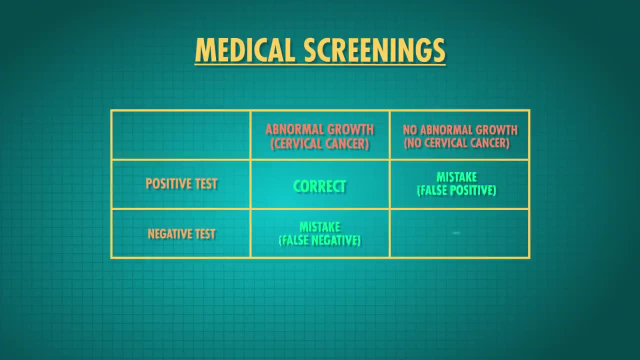 get screened once a year, But sometimes the results of the screenings are wrong. Either they can say there's something wrong or they can say there's something wrong, And that's what we're looking for. We're looking for something abnormal when there isn't. that's called a false positive. 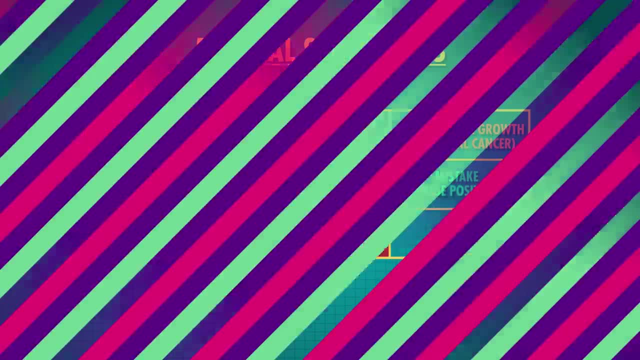 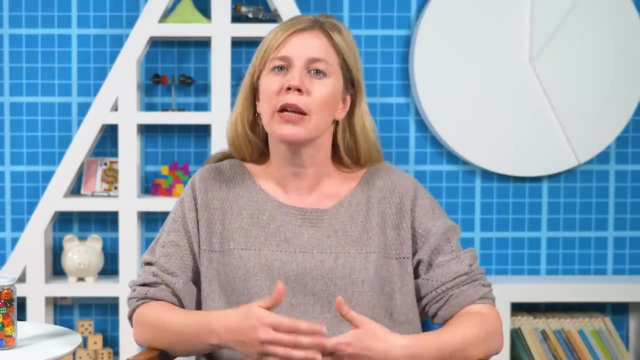 or that everything is all clear when it's really not called a false negative. This is exactly the kind of scenario where knowing the likelihood that something is actually abnormal, in this case cervical cancer, given that you've gotten positive test results, would be useful. 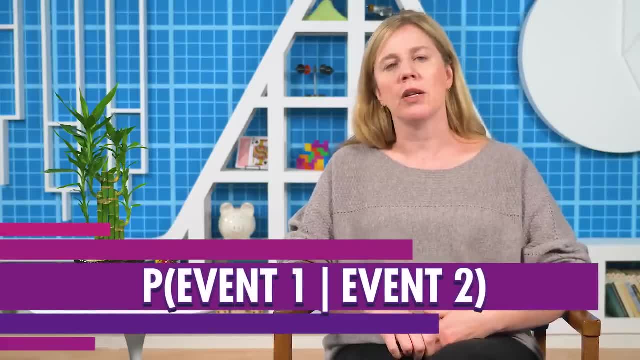 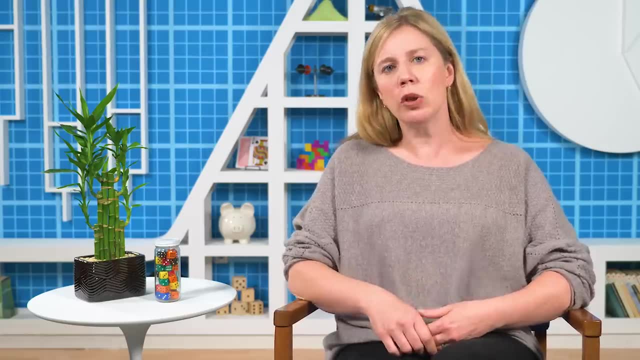 We write conditional probabilities as P of event 1, given event 2.. Conditional probabilities tell us the probability of event 1, given that event 2 has already happened. If two events are independent, like Cole and ice cream night, then we expect P of Cole, given ice cream night. 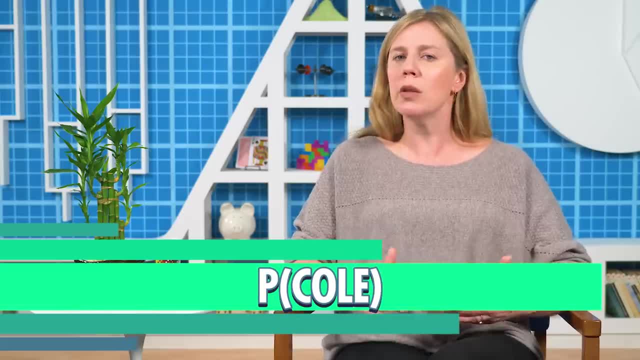 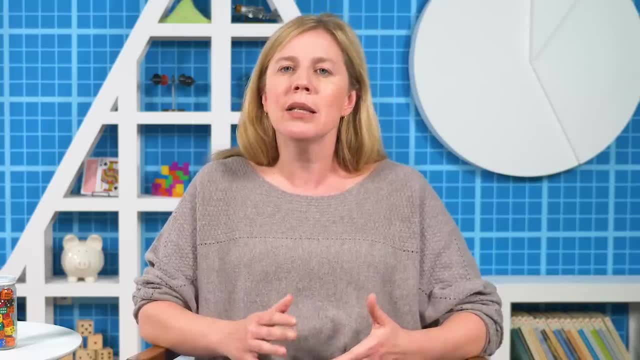 to be the same as just plain old P of Cole, since the two things are unrelated. If P of Cole given ice cream wasn't the same as plain old P of Cole, that means that ice cream night might somehow affect Cole's decision to show up at IHOP. 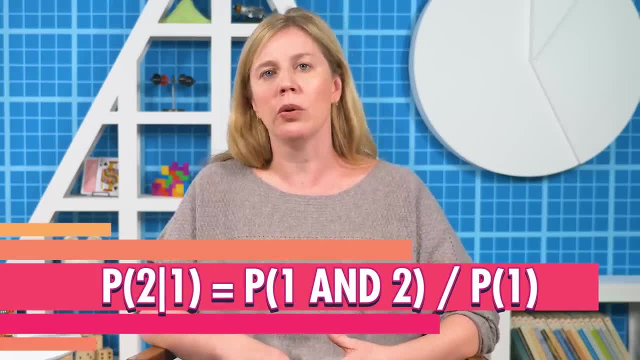 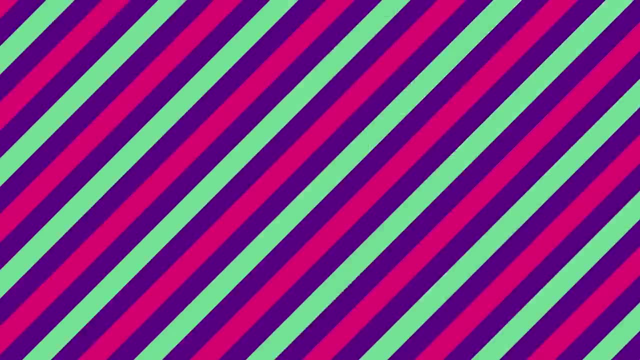 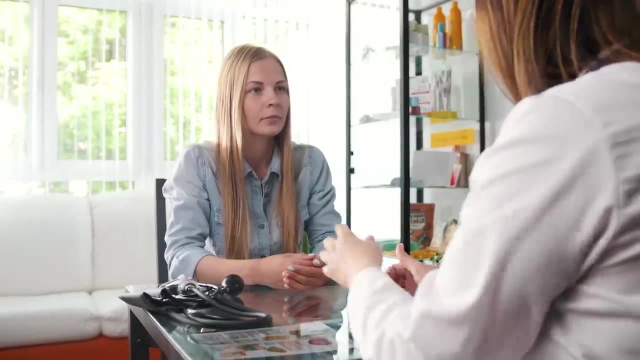 We calculate conditional probability P of event 2- given event 1, by dividing the probability of event 1 and event 2 by the probability of event 1.. The role of conditional probabilities are particularly important when we consider medical screenings, For example when screening for cervical cancer. 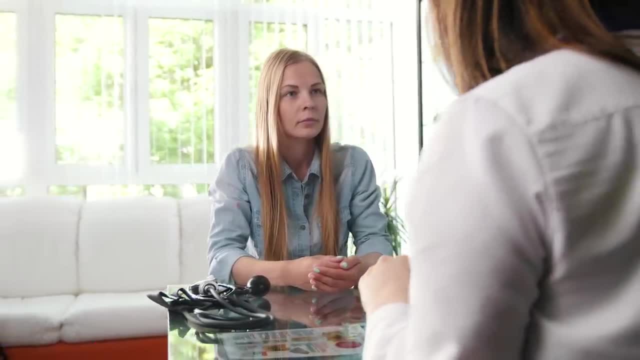 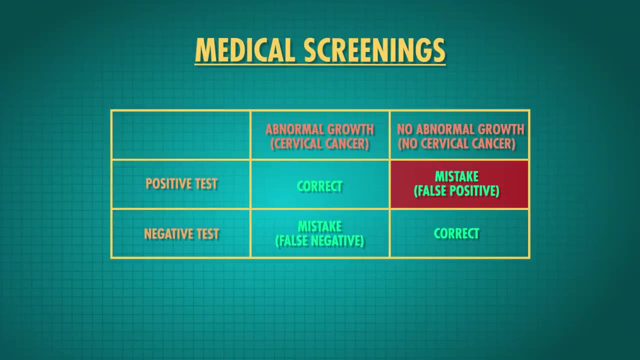 it used to be recommended that all adult women get screened once a year, But sometimes the results of the screenings are wrong. Either they can say there's something abnormal when there isn't, that's called a false positive, or that everything is all clear. 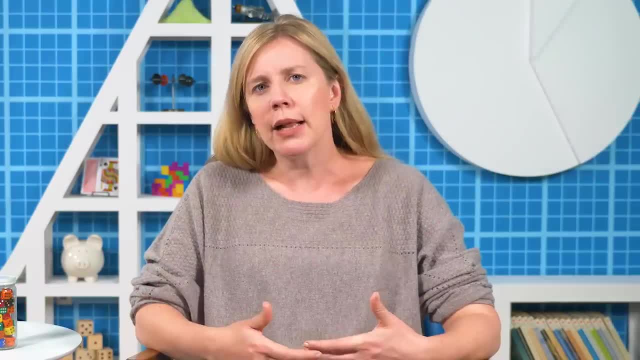 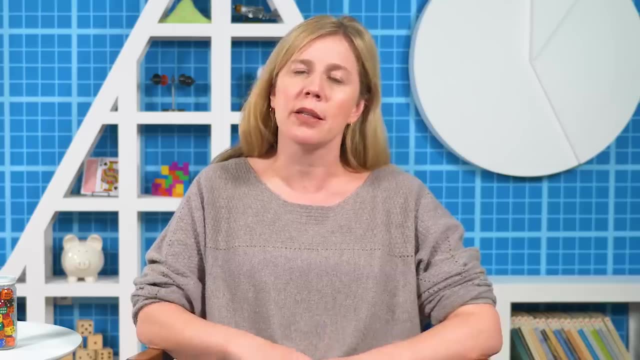 when it's really not called a false negative. This is exactly the kind of scenario where knowing the likelihood that something is actually abnormal- in this case cervical cancer- given that you've gotten positive test results would be useful. That is, P of cancer given positive test. 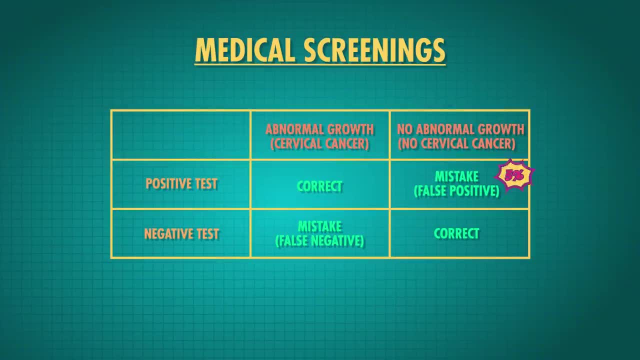 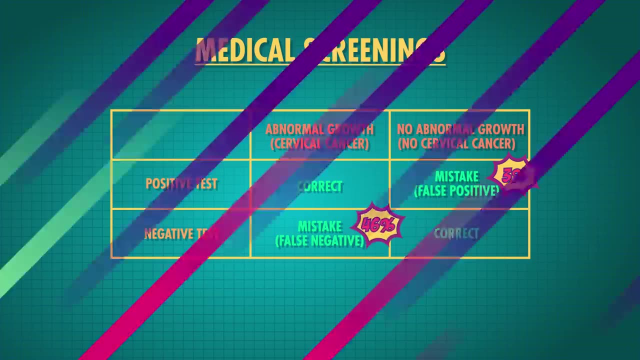 When looking at the data of people who don't have cancer, 3% will get a false positive And people who do have cancer will get false negatives 46% of the time. This means we miss a lot and maybe freak some people out. 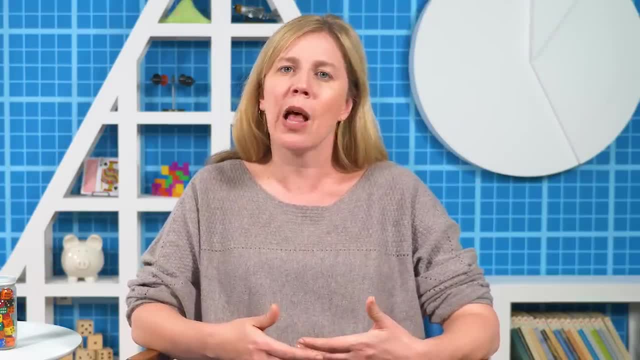 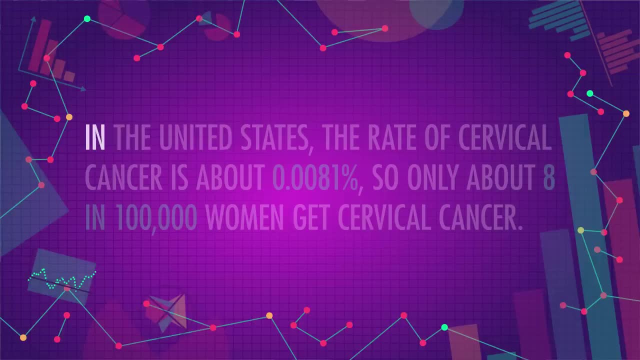 who don't need to be freaked out. The logic of conditional probabilities can help us make sense of why doctors have recently recommended that these tests be done less frequently in some cases. In the United States, the rate of cervical cancer is about .0081%. 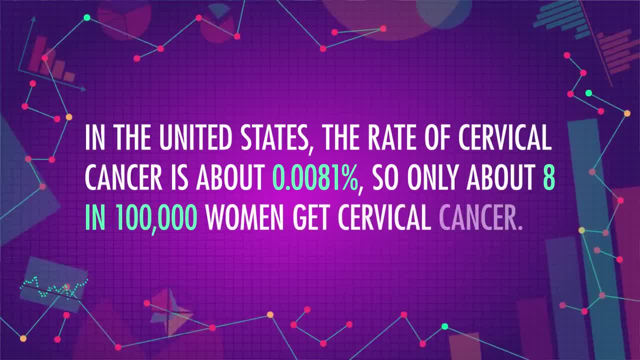 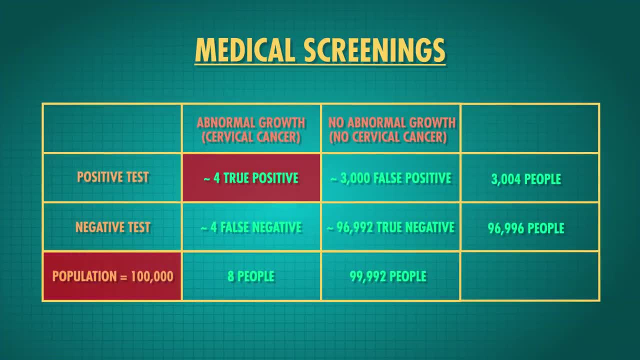 So only about 8 in 100,000 women get cervical cancer. Using our rates of false negatives and positives, we can see that 100,000 women in the US only about 4, of the about 3,004 people with positive tests. 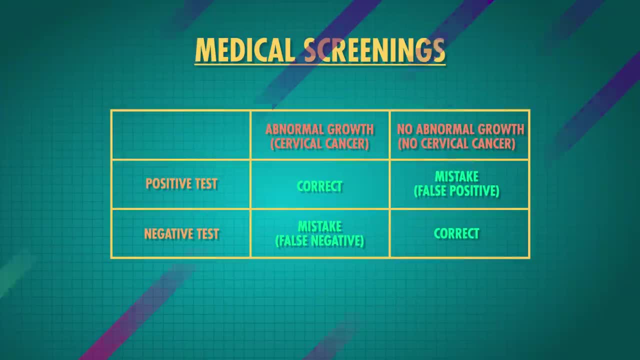 That is, P of cancer given positive test. When looking at the data of people who don't have cancer, 3% will get a false positive And people who do have cancer will get false negatives 46% of the time. This means we miss a lot and maybe freak some people out who don't need to be freaked. 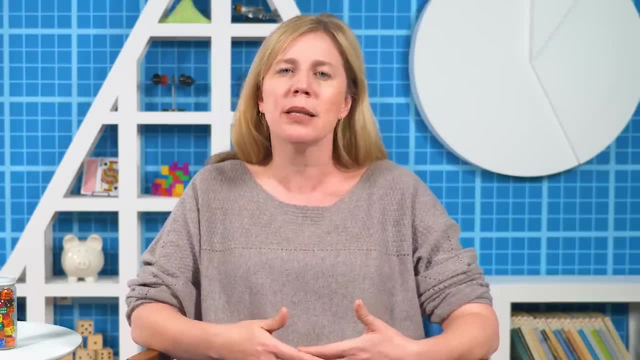 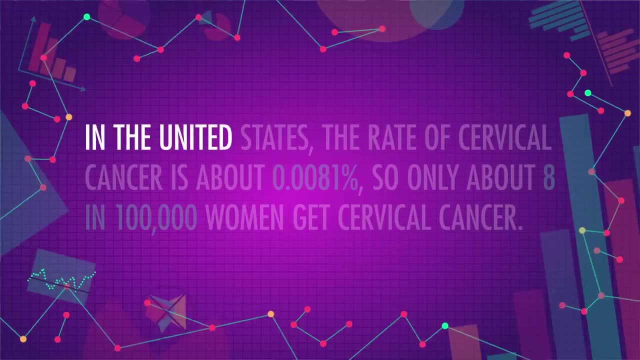 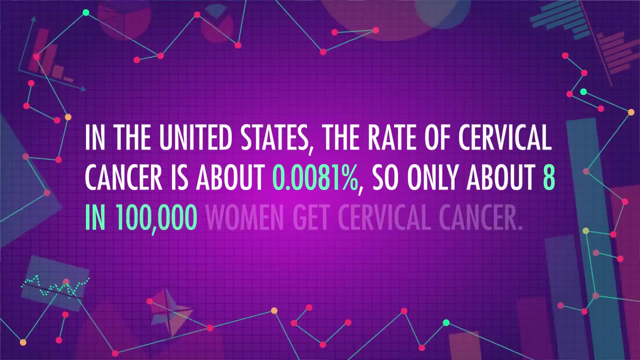 out The logic of conditional probabilities can help us make sense of why doctors have recently recommended that these tests be done less frequently in some cases. In the United States, the rate of cervical cancer is about .0081%, So only about 8 in 100,000 women get cervical cancer. 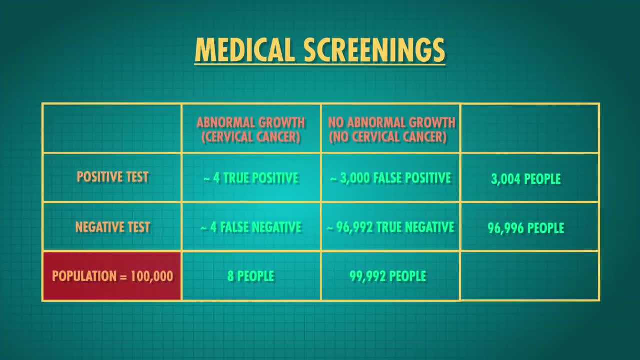 Using our rates of false, negatives and positives, we can see that for every 100,000 women in the US, only about 4, and we are rounding here- of the about 3,004 people with positive tests actually had abnormal growth. 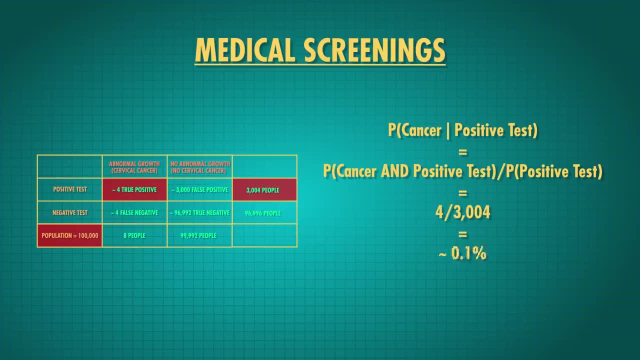 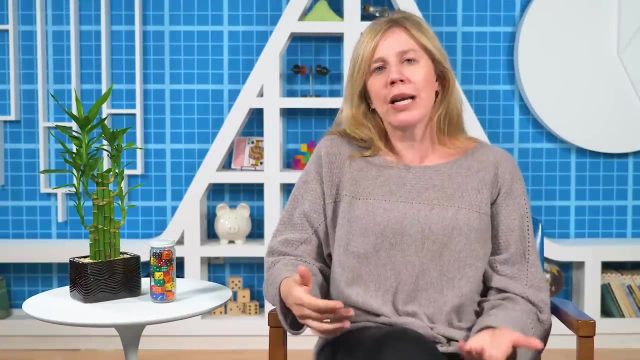 That means the conditional probability of having cancer, given that you've got a positive test, is only .1% Give or take. We're rounding And these positive tests require expensive and invasive follow-up tests, And I want to point out here that conditional probabilities aren't reciprocal. 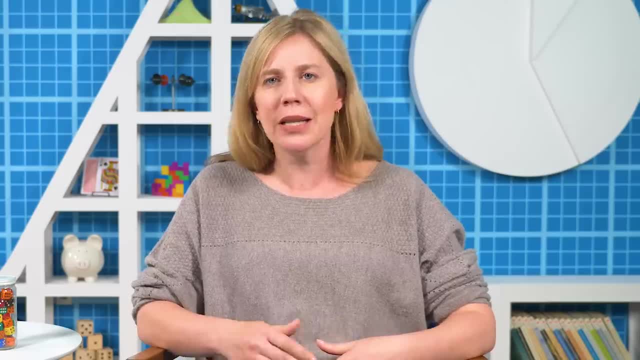 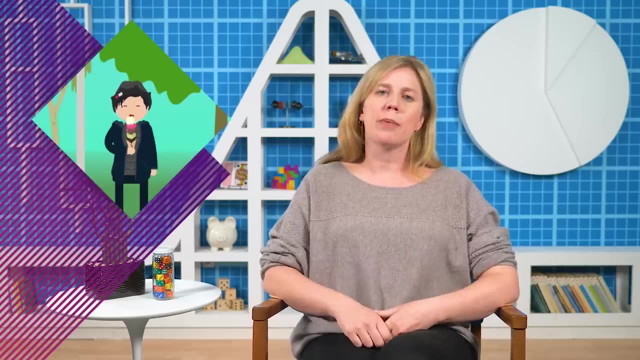 That is to say P of cancer given positive test isn't the same as false negatives. So we can't be sure The probability of having cancer isn't the same as P of positive test given cancer. That's about 50%. In real life you're not always going to know the probability of Cole Sprouse showing 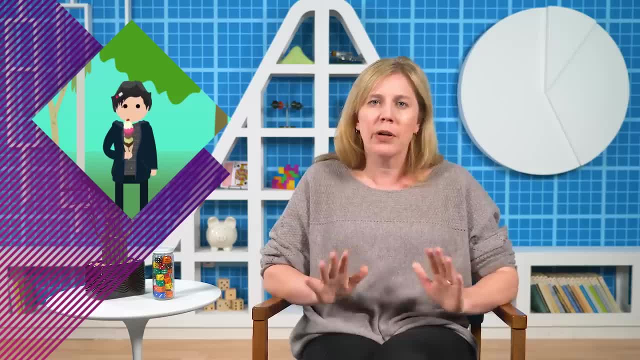 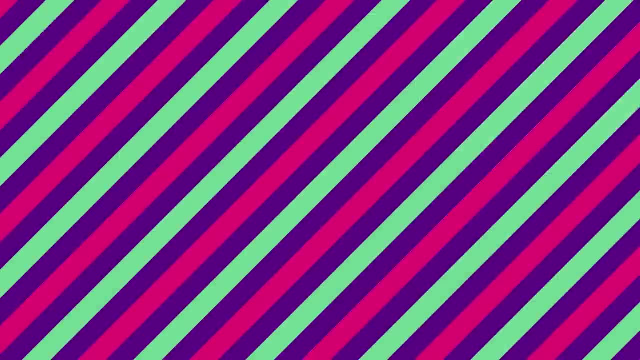 up at the IHOP. He's more unpredictable than I gave him credit for- Unpredictable like pretty much the rest of life. It can be really difficult to put a specific probability on a lot of everyday situations, Like how likely it is that your teacher will call in sick today. 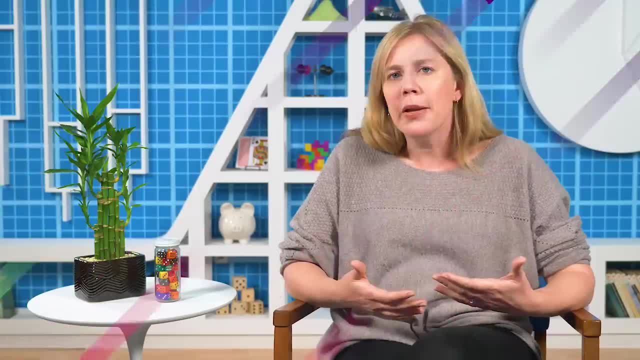 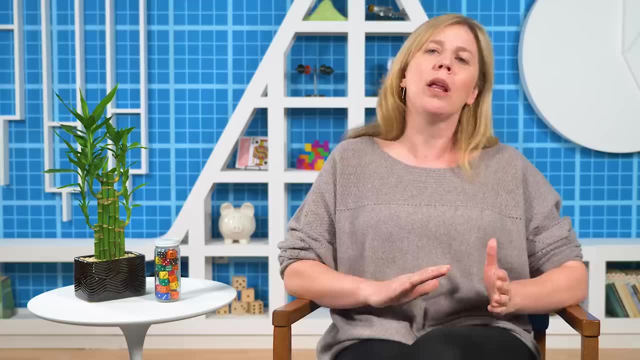 Like whether or not you're going to catch all the red lights on your way to school. Probabilities can, as we've seen, require a lot of calculations And there's not always time for that, But that doesn't mean they belong only on the school side of your brain. 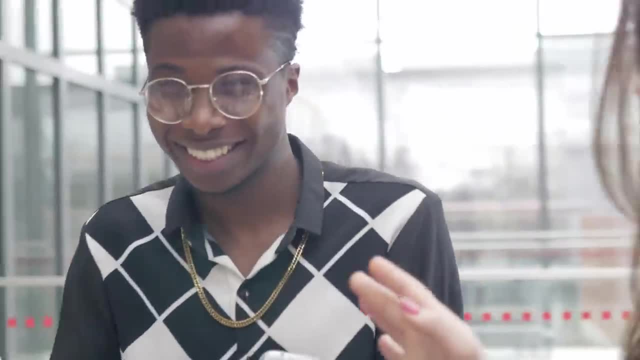 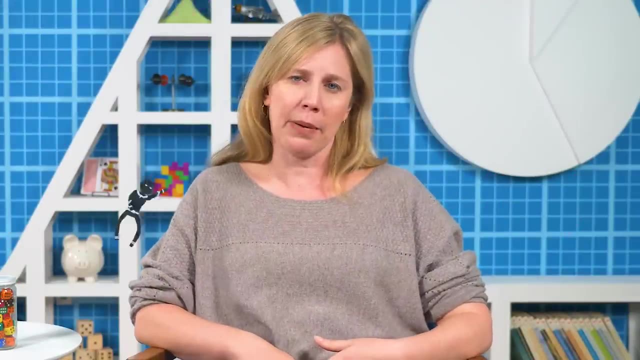 Say you want to go out on Friday night with friends. More than anything, you don't want it to suck. Last week you wound up on the couch watching Sandy Wexler again. You know it'll be hard to get tickets to see Black Panther, so you make a backup plan. 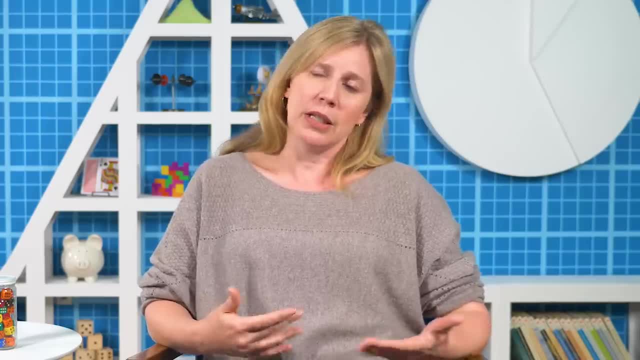 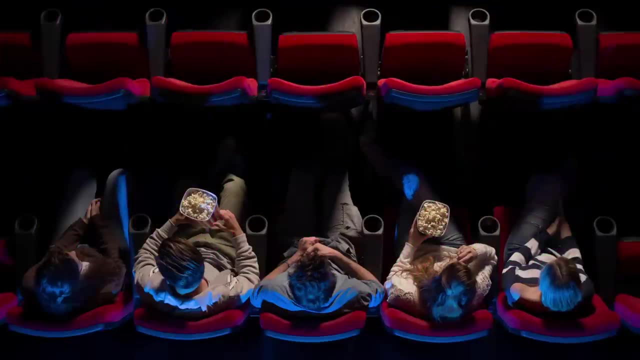 just in case You could always stream, Get Out Without stealing it, of course, But if you're determined to see Black Panther in the theater, probability will help you set your expectations. If you'll only settle for school, That's a good thing. 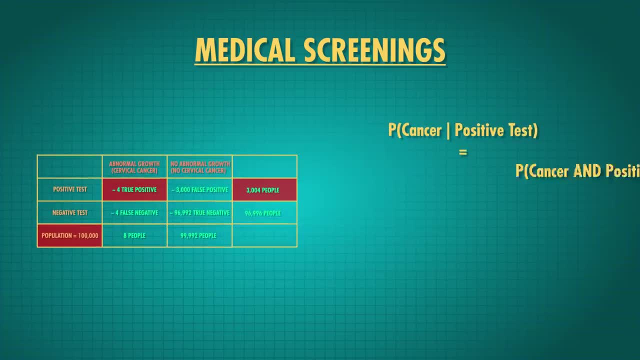 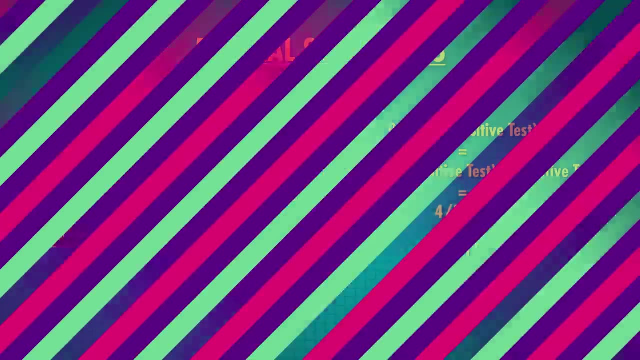 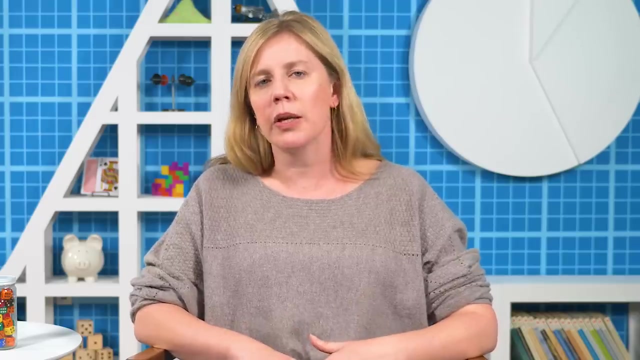 actually had abnormal growth. That means the conditional probability of having cancer, given that you've got a positive test, is only .1% Give or take. we're rounding And these positive tests require expensive and invasive follow-up tests, And I want to point out here that 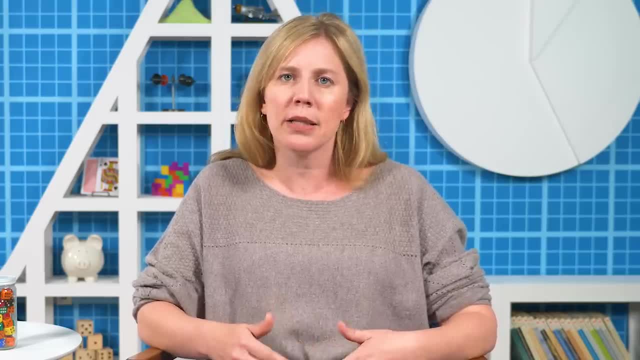 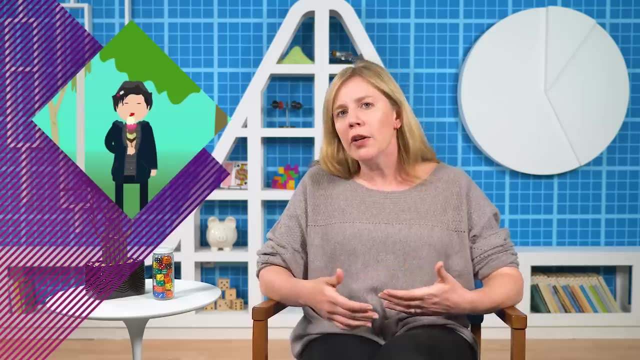 conditional probabilities aren't reciprocal. That is to say, P of cancer given positive tests isn't the same as P of positive tests given cancer. That's about 50%. In real life you're not always going to know the probability of Cole Sprouse showing up at the IHOP. 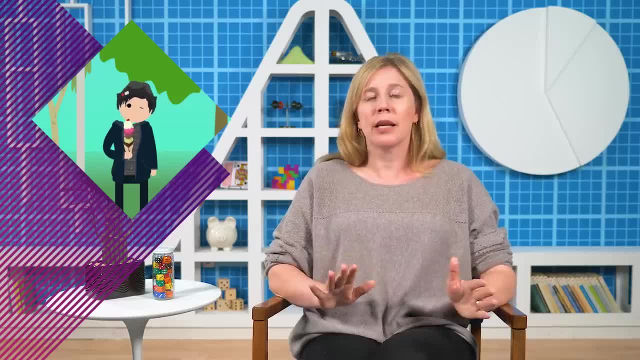 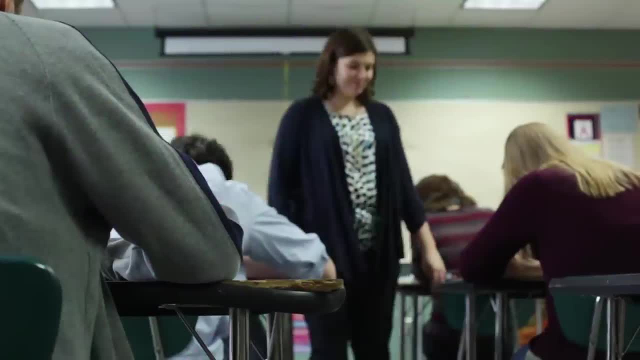 He's more unpredictable than I gave him credit for Unpredictable, like pretty much the rest of life. It can be really difficult to put a specific probability on a lot of everyday situations, Like how likely it is that your teacher will call in sick today. 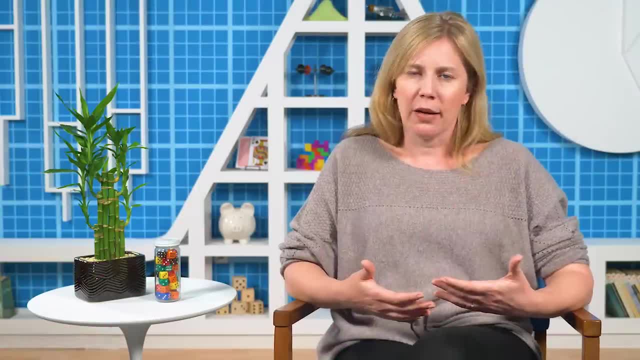 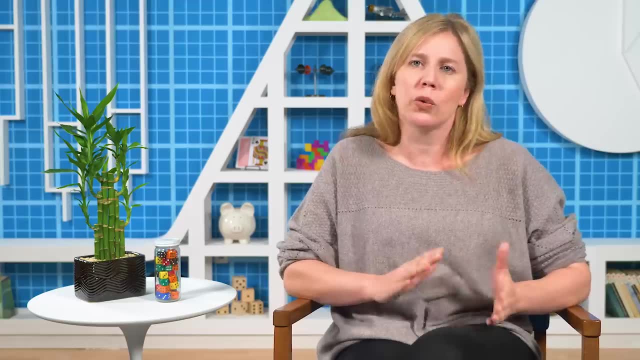 Like whether or not you're going to catch all the red lights on your way to school And, as we've seen, require a lot of calculations And there's not always time for that. But that doesn't mean they belong only on the school side of your brain. 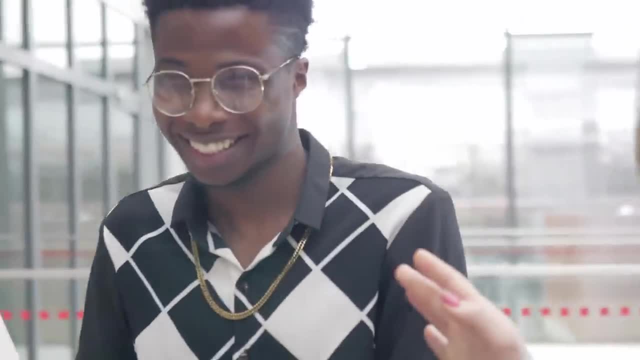 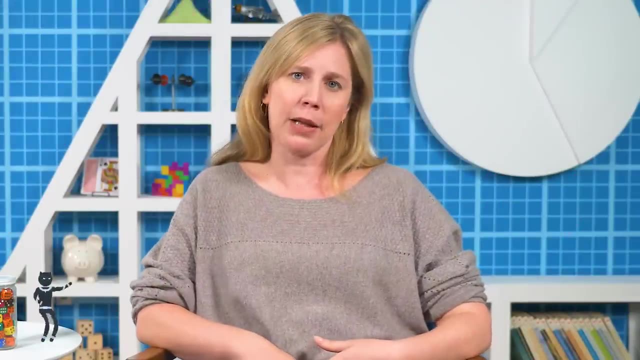 Say you want to go out on Friday night with friends. More than anything, you don't want it to suck. Last week you wound up on the couch watching Sandy Wexler again. You know it'll be hard to get tickets to see Black Panther. 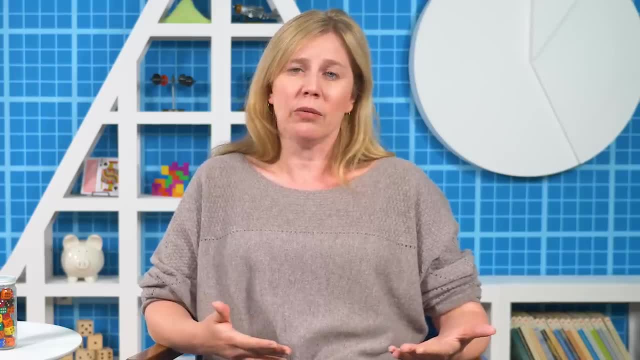 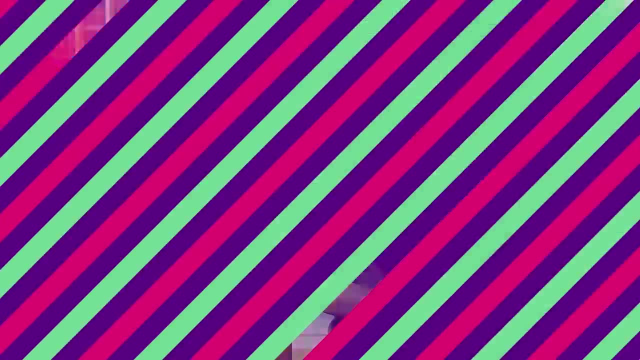 So you make a backup plan, just in case You can always stream, Get Out without stealing it, of course. But if you're determined to see Black Panther, probability will help you set your expectations. If you'll only settle for center row tickets, you're more likely to be disappointed. 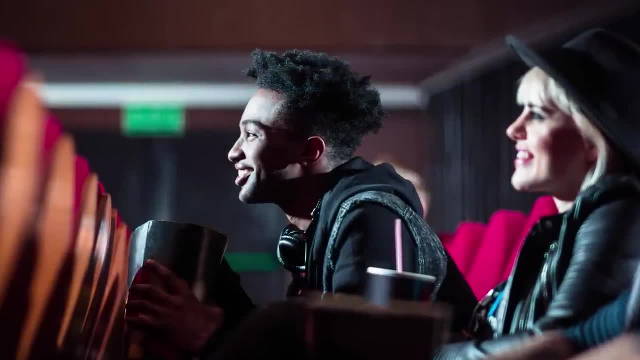 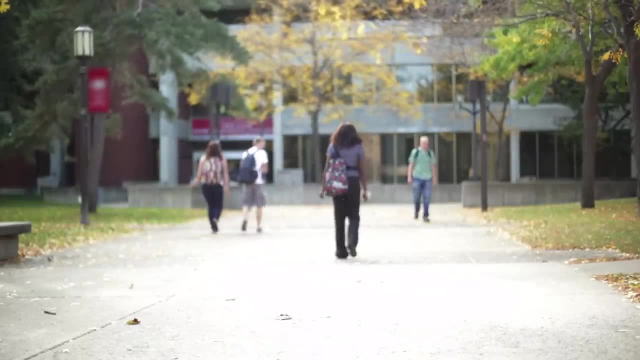 Your chance of seeing Black Panther is going to be greater if you're willing to settle for whatever tickets you can get. Probabilities help us understand why it makes sense to apply to more than one college, Why you shouldn't expect that the first short story you write